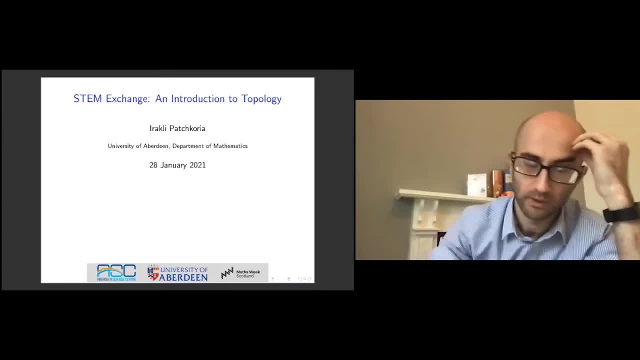 talks for now. I'm a mathematician, but not for, like, non-mathematicians, So I apologize in advance if this doesn't really go up to your standard you are used to. So, yeah, but let's see. So here is an. 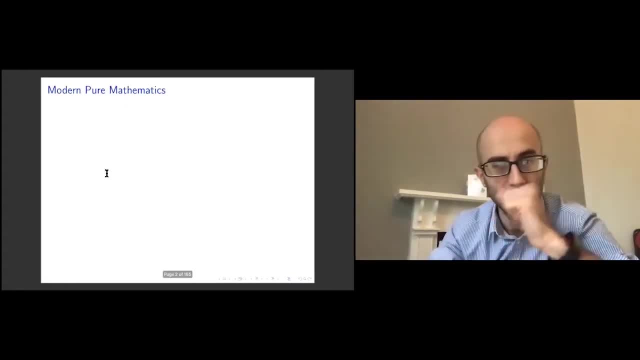 introduction to topology. Let's start with discussing generally what the modern pure mathematics is doing, and I mean it's a huge subject with many different areas, and some of these areas you might have heard names of. Let's just mention them Before we really go to topology. so one of them is analysis, which is 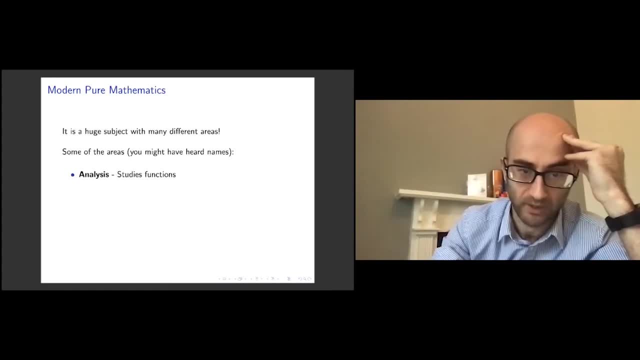 something that studies functions, and you might remember what these are from your school. Then there is algebra and number theory, which kind of studies numbers or equations, and then something which is relevant for us today is geometry and topology, which studies figures, geometric objects, distances, shapes, and now 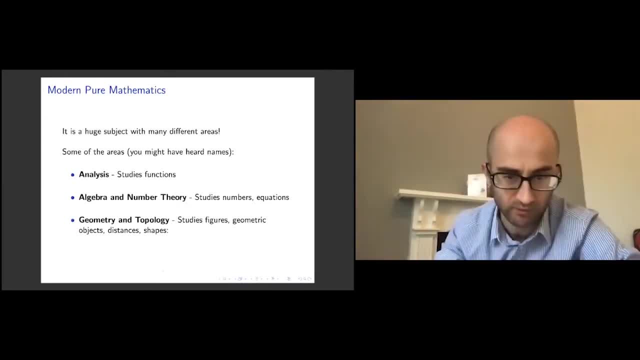 I mean, you might think that this guy is going to keep on now writing this kind of text on the slides, but most of the time, what we will be doing in this talk will be looking at pictures. so let's start looking at some pictures. so we switch now to geometry and topology. so geometric objects. 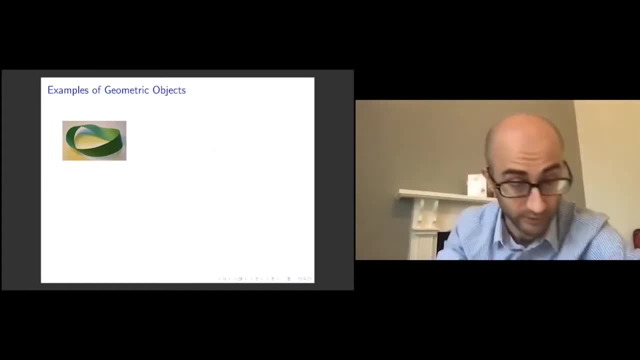 examples of geometric objects. I mean here, for example, this is this famous Möbius band which we will discuss shortly, here is a sphere, here is a torus, these kind of things. So here we have the things should be familiar in, uh, for many people here. then we got here something very similar to: 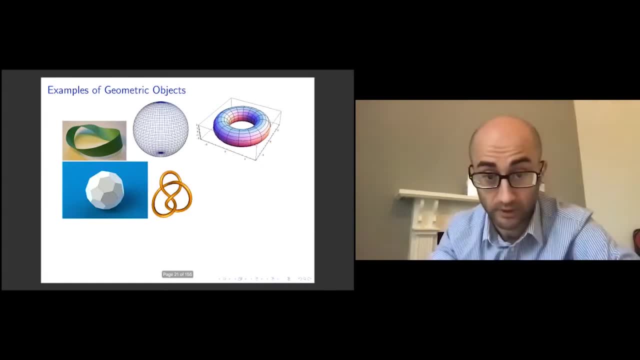 football ball- not quite a ball because it's not round. here is a knot. this is a klein bottle- again something you might have seen in some popular science talks. and then, all in all, uh, these things are some things we can still kind of imagine. but now we start here seeing. 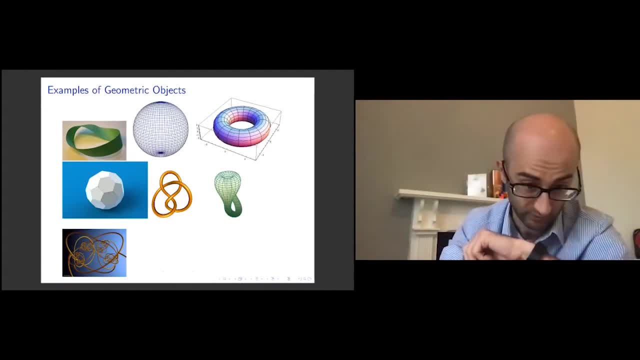 some outrageous geometric objects. this is something called alexander's horn sphere, that's a columbia threefold and that's a three-dimensional sphere. so these are things that are not quite really- i mean these last two- not quite really- sitting in three-dimensional world, but i will still mention at the end of this talk what they. 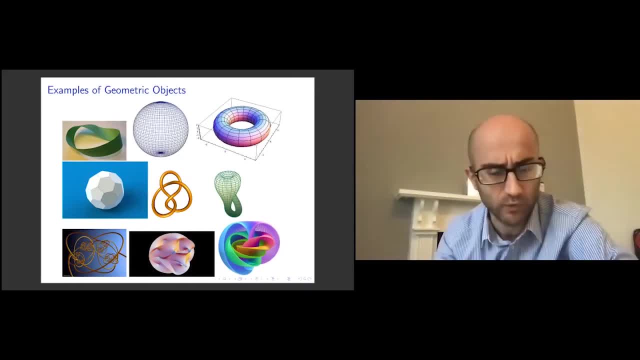 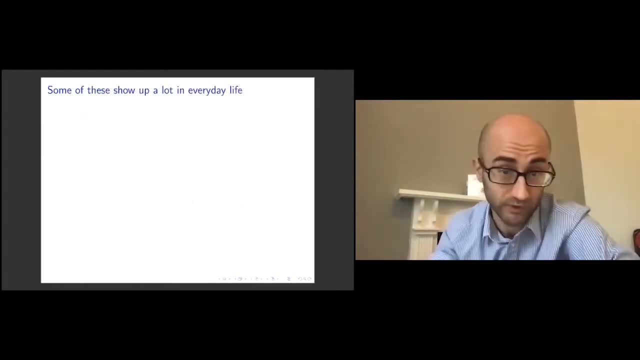 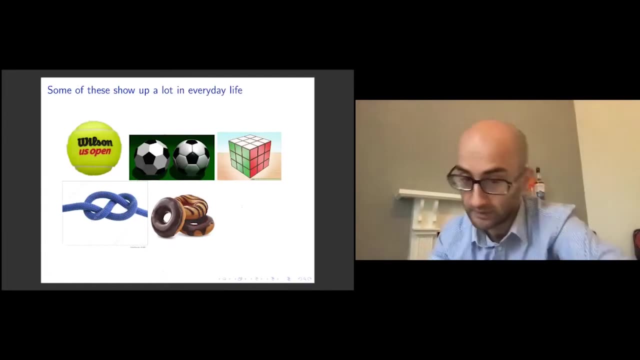 really are okay. so now, uh, looking at these objects, of course some of them are objects from real life, like these things here, for example, we meet them. some of these things, we meet them in everyday life, like, look at these things, picture, for example, like football ball or donut or a knot, these things, of course, show up in everyday. 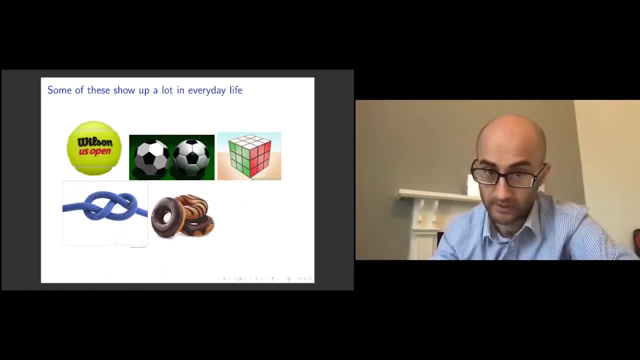 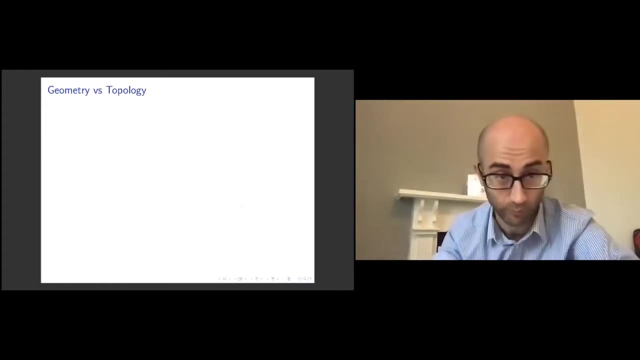 life. so, in that sense, studying those objects here is nothing crazy. i mean, these are really things in real life, and and and we have to study them. okay, so now, what's the difference between geometry and topology? so, as i said, this talk is about topology, so maybe we should first explain what's the 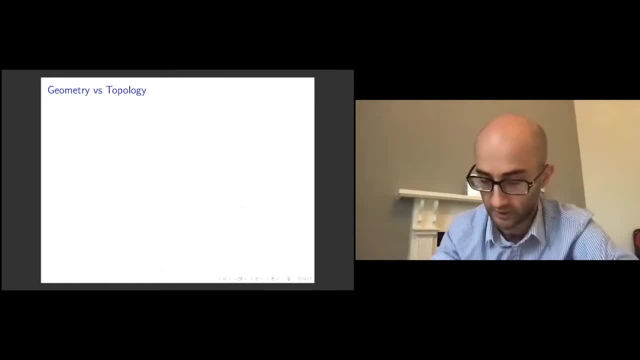 difference between these two subjects. i mean, this is a very naive explanation. again, many people might argue against this uh reasoning, what i will do here, but anyways, geometry is something that often studies metric properties of geometric objects, so like shortest distance between points, or measures or volumes, and, and these are kind of things like more like quantitative kind of things. 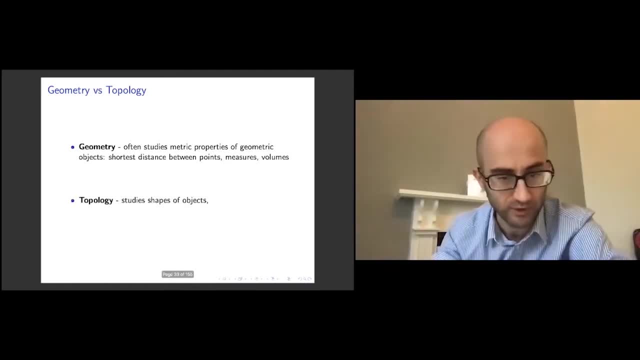 that's what geometry very often studies, whereas a topology this is concerned more about shapes of objects. you know how they look like and what are the characteristic properties of these shapes, as opposed to how exactly large they are or what's the volume of something. so really interested in the characteristic properties of these shapes, and so this talk. 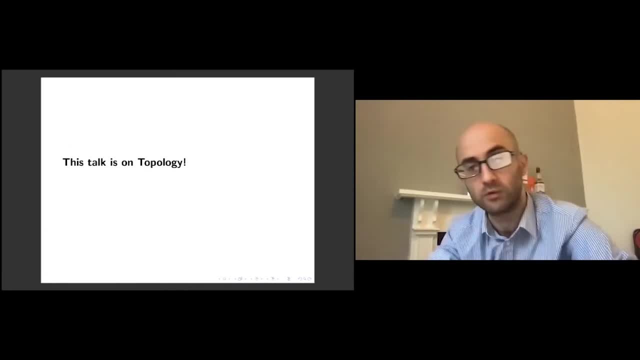 is on topology, so this talk is in topology and and what i want to show you is the first example of such a characteristic property, such a topological property which you can observe on something, something, something, something, something. you can look at a part of the image where you could see ordered. 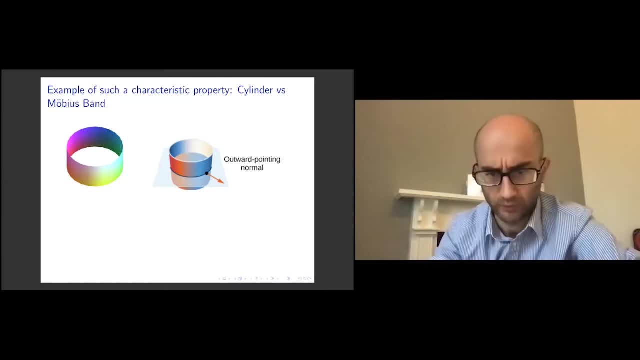 the depication of. so hold on, can you take out the table pointing arrow on this black point When this black point is running around? imagine this black point is a bug or something that is running around along the circle. While running around the circle, this arrow will keep points outwards, you know. and then, once this point starts moving, 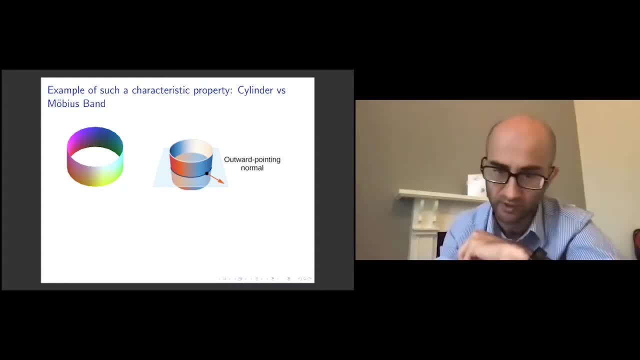 around and it comes back to the same spot. this arrow will come back to itself. I mean, this is pretty easy to imagine if you see the shape of the cylinder. But then there is this cousin of cylinder which is called the Moebius band, And this Moebius band has this kind of a shape. 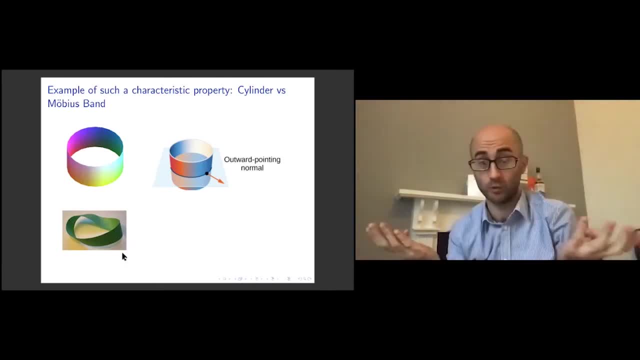 And this shape can be also obtained by gluing: taking a piece of paper and gluing two sides, but by a twist, And now this Moebius band has this property- that if you start with an arrow at this spot here and you try to do the same thing and you let this point run around in the 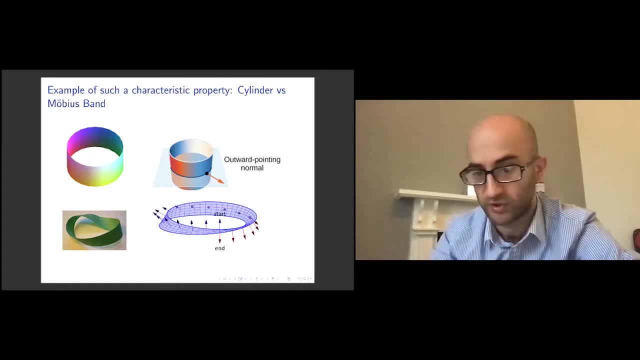 middle of this surface, then you come back to the same point And then this arrow will point in a different direction. So, and that's sort of the qualitative characteristic difference between these two shapes And this property really distinguishes them, And that's what topology is about. So you give me two objects and I find one property. 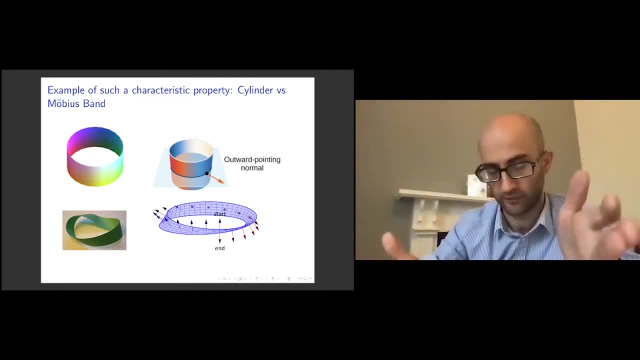 and then I find another property And these two properties are different for these two surfaces. so I conclude that they are different, And this property in topology is called orientability. for example, This tells you that the cylinder is orientable, whereas Moebius band is not Okay. so this was just a warm up, you know. 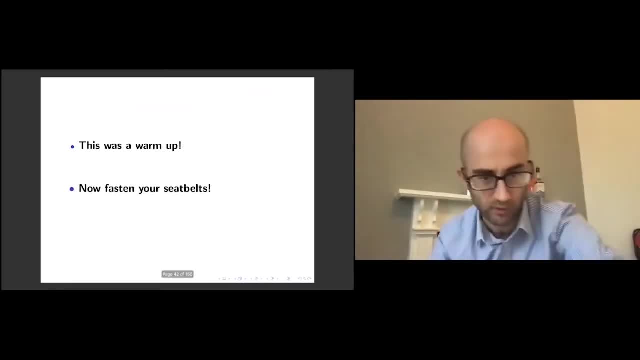 to show you what kind of properties we will care about. So now you should fasten your seatbelts, because things are going to get a bit more complicated. No, I'm joking. So now we're going to start with looking at pretty easy objects, And these objects are beautiful objects. 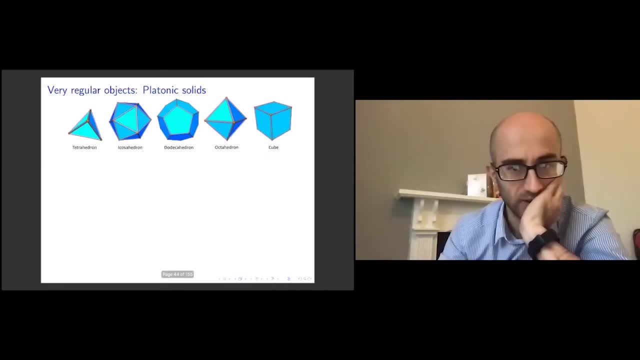 very regular objects called platonic solids. And so here is the list of platonic solids: tetrahedron, icosahedron, dodocahedron, octahedron and cube, And one of the goals of this talk is to show you that these are the only ones in certain sense, And 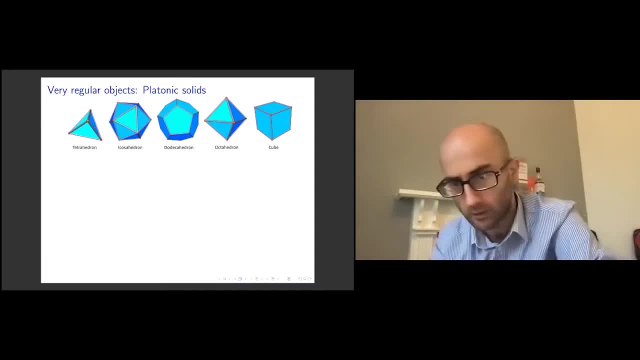 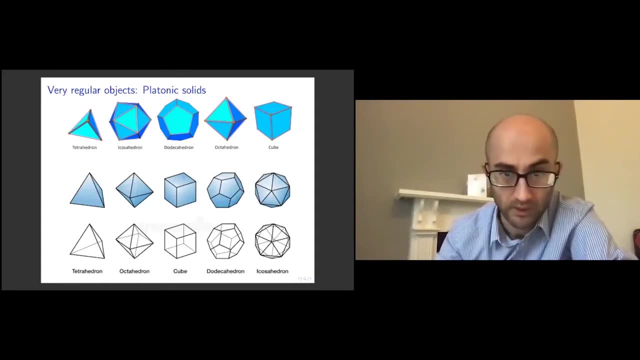 this was already kind of known by Plato in old Greece. All right, so another way of looking at them if you have never seen these objects. and now I should tell you what these are. So what are the platonic solids? First of all, they are polyhedra. 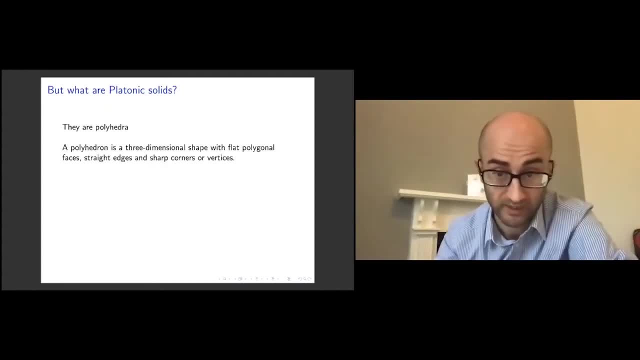 So a polyhedron is a three-dimensional shape with flat polygonal faces, straight edges and sharp corners or vertices, Like. if you don't understand this definition, at least look at these pictures. And these are the type of things that are polyhedra. So some. 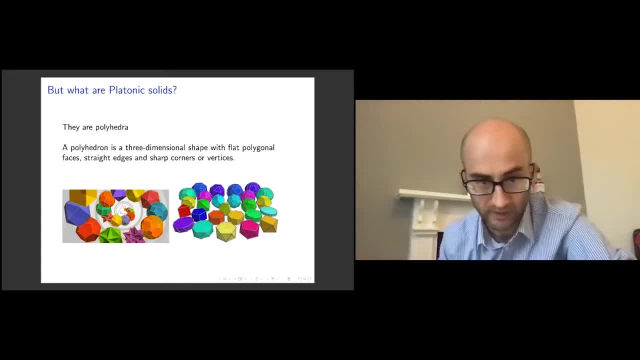 kind of shapes with flat faces and edges and corners, And you see that they come in many different types, Like, for example: here we have some of these star-shaped things, But obviously we don't have many of these and we want to get platonic solids out of them, So we need some. 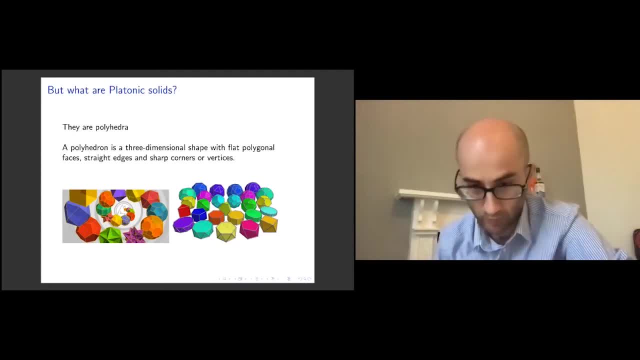 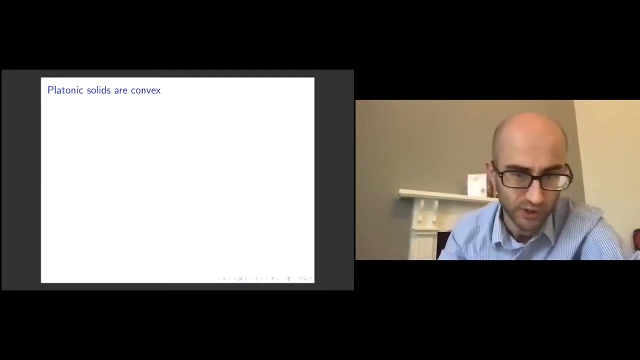 extra properties for these platonic solids satisfied in order to be able to distinguish them out of the rest of the world of polyhedra. So the first property with this platonic solid satisfies that they are convex. I don't want to really define what convex is officially Here. I 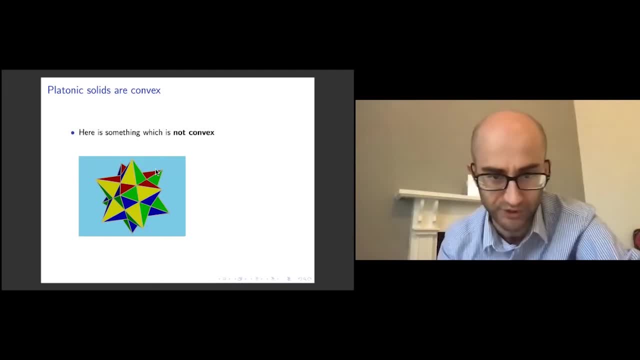 will show you something which is not convex. this picture: you see the star shaped surface here and this is an example of something not convex, And what does this really mean? If you take these two vertices here, for example, if you see, hopefully you can see my mouse, if you try to connect these two points with a straight. 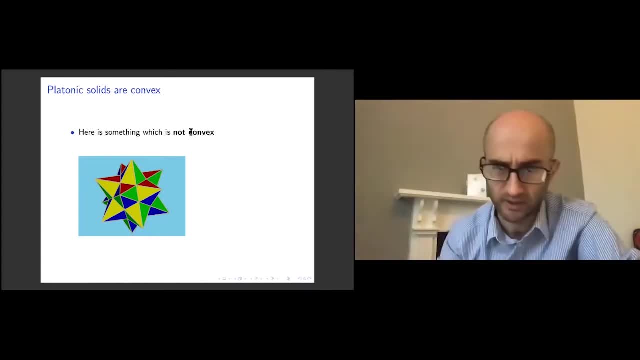 line, then you're going to go outside of this shape, And this means that this thing is not convex, Whereas platonic solids are, of course, convex, like the pictures you saw. those were all convex. So we definitely want convex polyhedra. So now topology studies, characteristic properties of 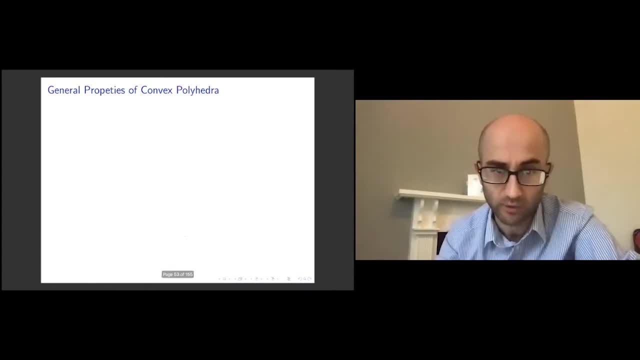 polyhedra, and it's one of the things it studies, And so let's investigate what are the general properties of convex polyhedra? And so here are the things that always come with a polyhedron. So every polyhedron has edges, faces and vertices. 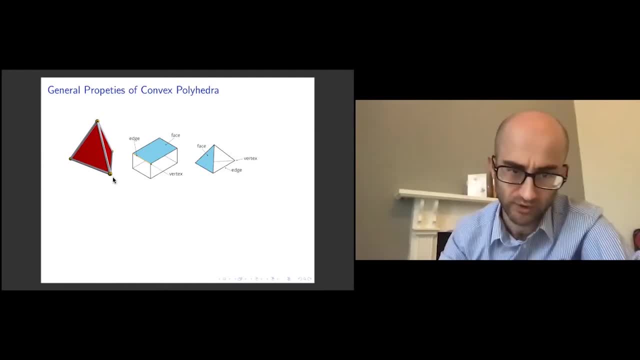 Like on this picture on the left, with the colors you see this: gold, gray and red. So the gold color, these are the vertices, these gold little points, these gray lines, these are the edges and the red things these are the faces. 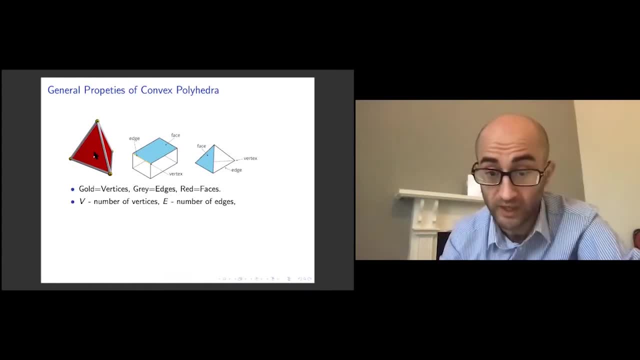 So I will denote by V number of vertices, by E number of edges and by F number of faces. And now, in this case, with a tetrahedron pyramid on the left or on the right, let's ignore this box for a second- V is equal to four. As you see, there are these four little gold points here. 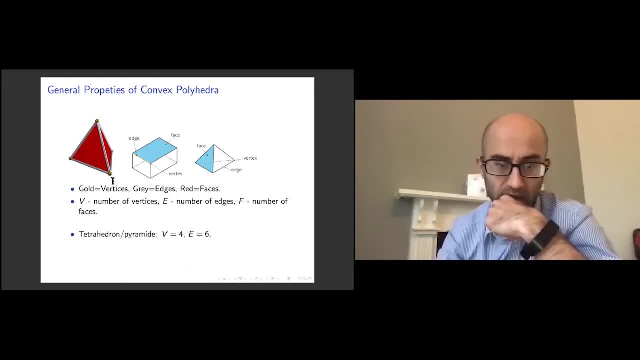 and that's four. E is equal to six, and that is exactly these gray edges here, what you see- And F is equal to four. So, like, if you look at this picture, there are exactly four faces. There's standing three triangles and the bottom triangle. Okay, but now what these things satisfy is that, if you 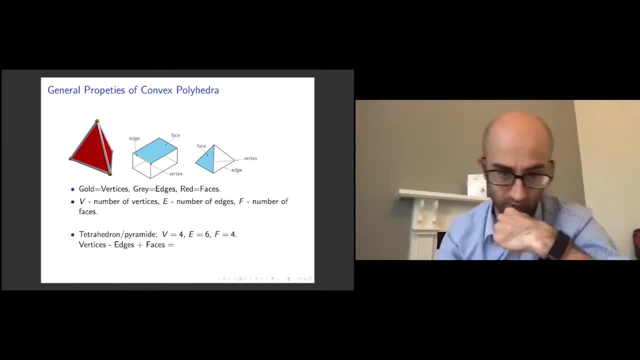 take vertices minus edges plus faces, so number of vertices minus number of edges plus faces, which is V minus E plus F. Let's see what happens in this example. I mean most of you hopefully remember calculations in the school- Four minus six plus four is equal to two. 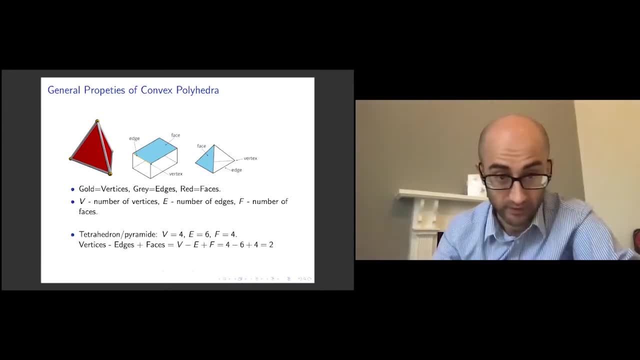 Everybody can compute that right. Great. And it turns out that if you do the same thing for this box, which I don't want to write down now again, this V minus E plus F will be equal to two. Okay, so is this a coincidence? Let's look at another example. 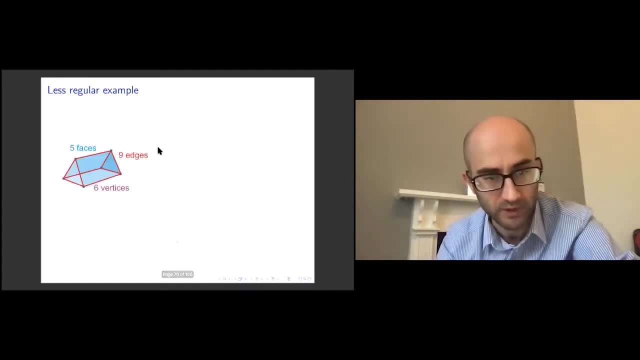 less regular example, For example, such a thing. This is definitely not a regular polyhedron, but it's still pretty good looking polyhedron. So here you have six vertices, nine edges and five faces, Like on the picture. the violet ones are vertices, the red ones are edges. 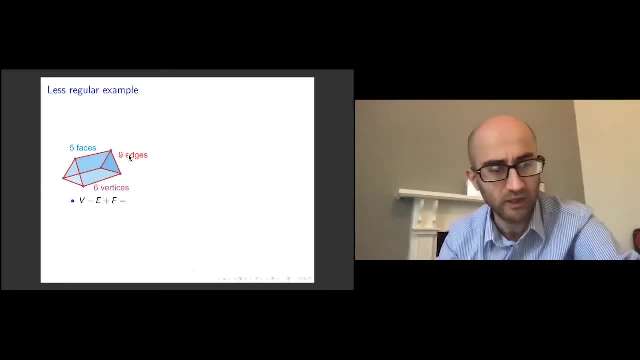 and blue ones are faces. And again you take V minus E plus F, so vertices minus edges plus faces. This case it's six minus nine plus five. So let's do this computation. I mean, everybody can do this again in this audience. I hope That's equal to two again, Wonderful So. 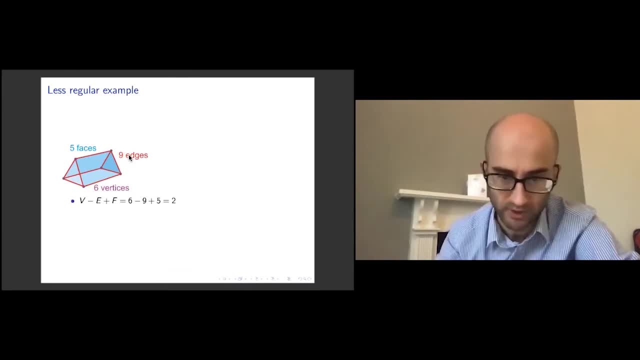 what's going on here. So it turns out that this is a general phenomenon, and this is often how mathematics works: You observe examples and then you guess that something should be true. And this guy called Leonard Euler in the 18th century, a very famous Swiss mathematician, one of the 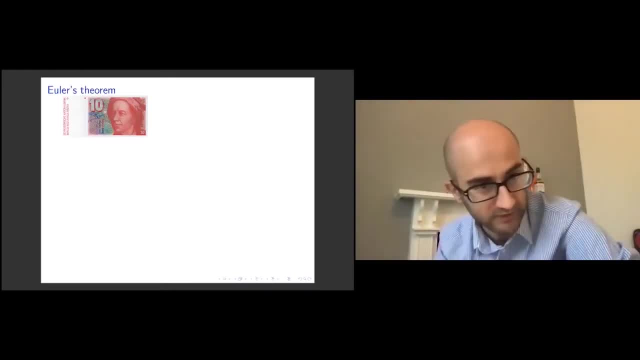 greatest mathematicians of all time, here shown on the banknote of 10 Swiss francs. this guy proved that for any convex polyhedron, if you take vertices minus edges plus faces, V minus E plus F, that is equal to two Always. And it turns out that this is a consequence. 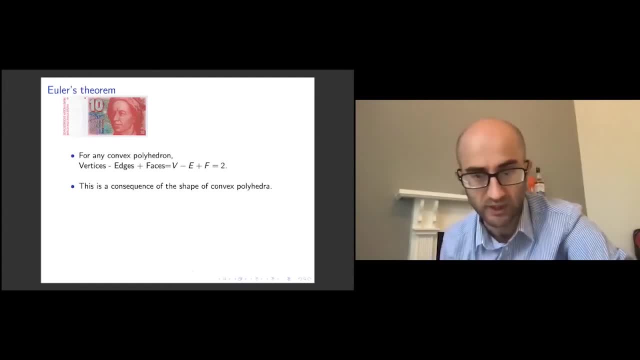 of the shape of a convex polyhedron. This is a consequence: how these convex polyhedra look like. It's their characteristic property, So it doesn't really matter how big they are. what are the lengths of these edges or how big these corners and the vertices are? I mean. 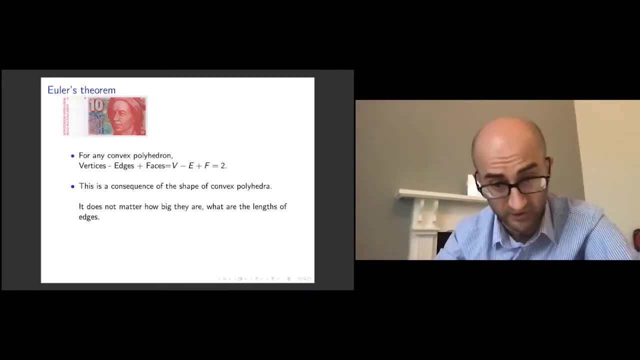 what really matters is just the shape of this convex polyhedron, and this is a characteristic property of that shape. So that's what kind of the properties topology is interested in, that particular shapes satisfy some properties, independent of how big they are. And just to mention, what does this have to do with modern maths? I mean, this expression is: 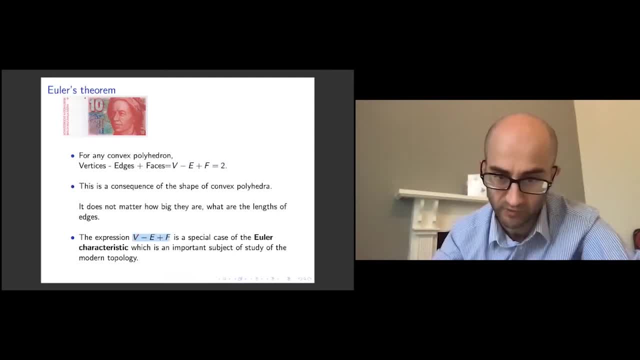 a special case. This V minus E plus F is a special case of something way more general called Euler characteristic, which is a very important subject of study of modern topology. Let me throw in here some buzzwords. It can be defined in terms of something called homology, And this homology is something that topologists 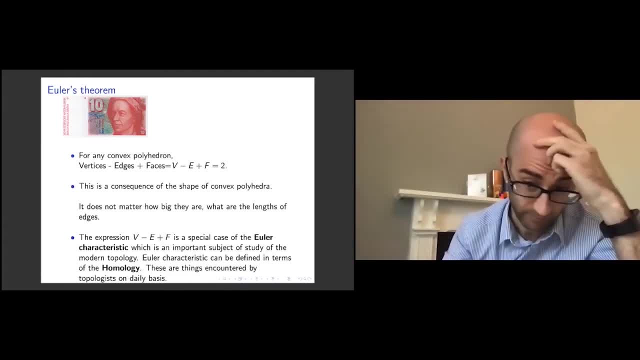 encounter on a daily basis. So, for example, I don't know, yesterday maybe I was computing something and I was using, I think, homology, for example, And maybe, oh yeah, yesterday I actually attended a talk which was doing some cool things with Euler characteristic. 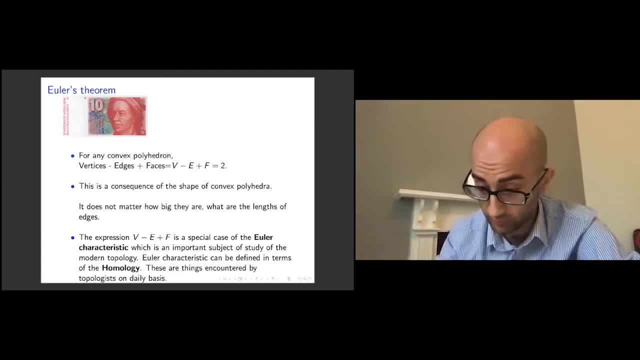 for example. So you know, this is very close to modern topology. It's just like it's a very, very special case of something which is more general in research. All right, so that's Euler's theorem. So why do we care? 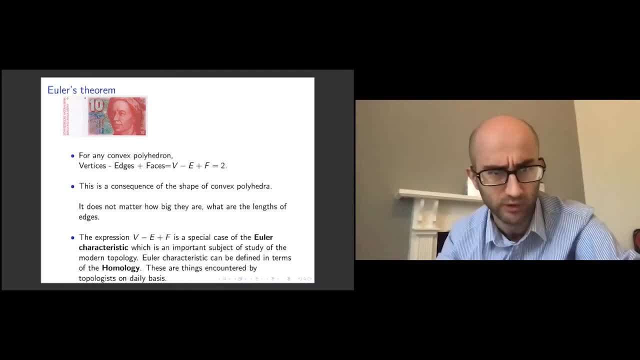 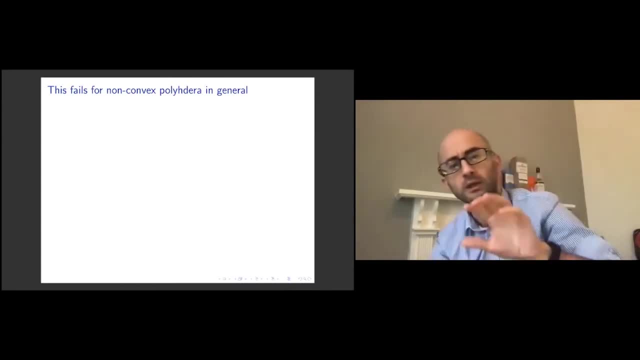 about Euler's theorem. So this allows us now to classify platonic solids. So, but before I tell you this, just to make a point, here I was talking about convex polyhedra. This property, this V minus E plus F, equal to two, fails for nonconvex polyhedra. And this 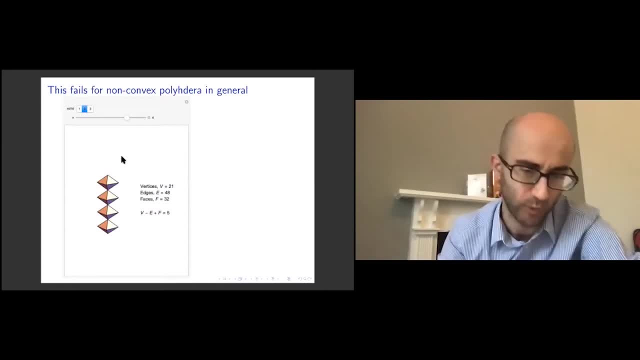 is an example like this: thing here is not convex, but it's a polyhedron. But if you look at this expression- vertices minus edges plus phases- in this case it's equal to five, not to two. So that equation was really characteristic for convex polyhedra. All right, So now we 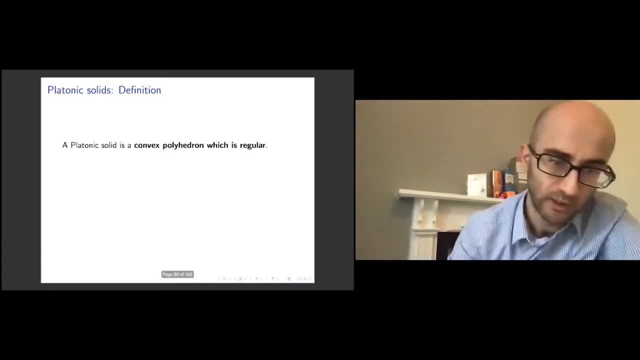 are ready to define platonic solids. So, given official definition, a platonic solid is a convex polyhedron, which is regular. So a convex polyhedron is regular if all faces are identical. regular polygons, all side lengths are equal and all angles are equal. So once, 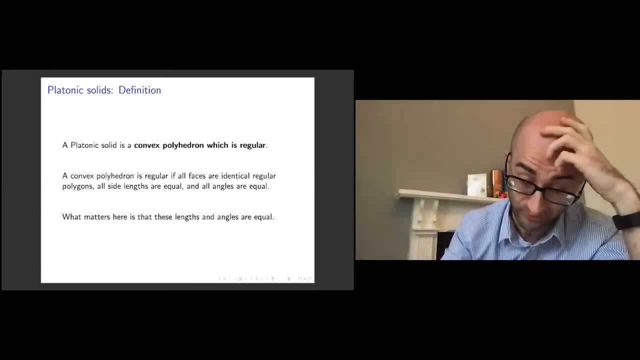 again, what matters here is that these lengths and angles are equal. It doesn't really matter how long they are or how large they are. So we are just interested in this qualitative property, characteristic property of this: lengths and angles, that they are equal. We 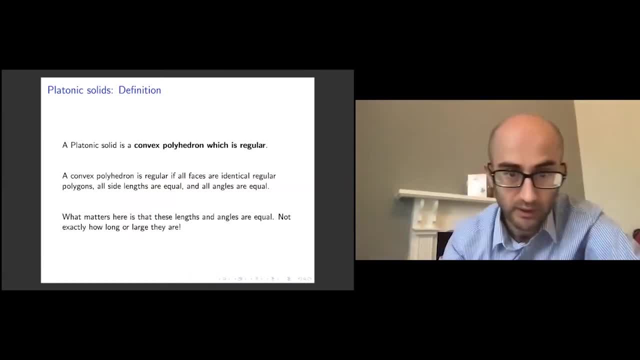 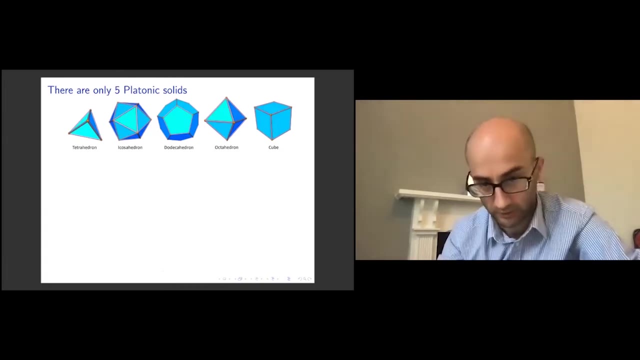 don't care how long they are or how big they are. So, and here is example. I mean, the claim is there are only five platonic solids, And let me show you how you do this. And here are all of them. And again, Plato was saying that these are all of them, but he couldn't prove it. Now 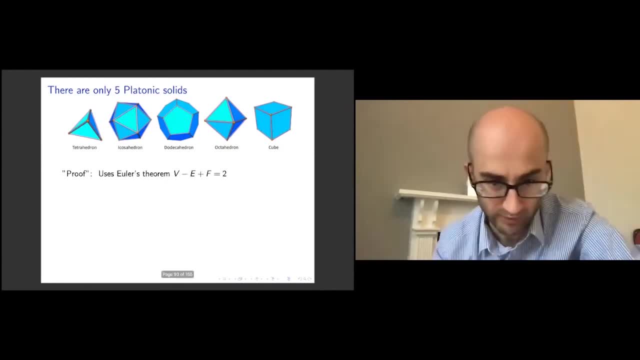 we can prove this. So, of course, we're going to use Euler's theorem, We're going to use this equation which we mentioned here, and let m denote the number of edges of each face. For example: here this is three because we have triangles. here, Here this is six because 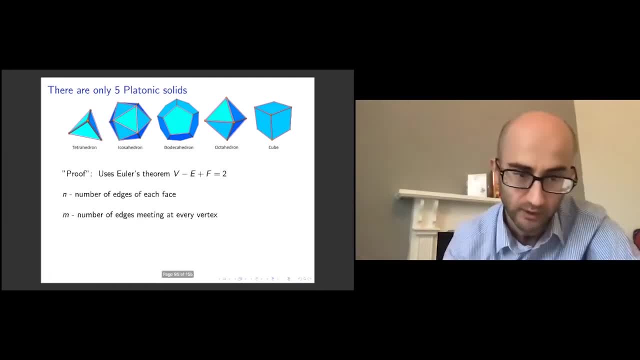 here we have a hexagon. Here it's four, because we have squares, And m denote the number of edges meeting at every vertex, Like in this case. it's three. In this case, I think, it's 1,, 2,, 3,, 4, 5.. In this case, it's 4, 1,, 2,, 3,, 4.. And 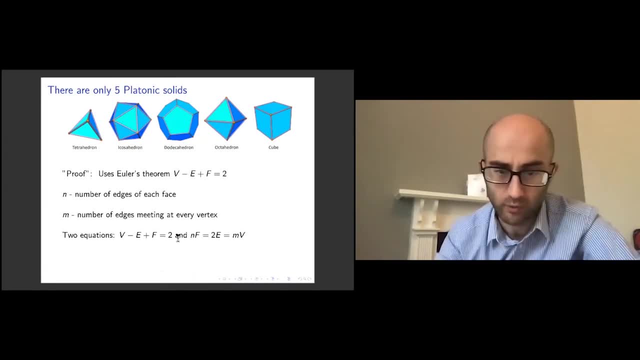 it turns out now that we have these two equations: One is Euler's equation And on the other hand we have this equation, which is a consequence of being regular. I don't want to go into like how this equation now follows, But anyway. so we do know that every platonic solid should. 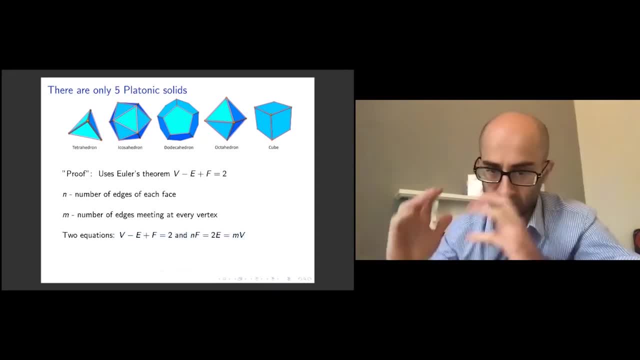 satisfy these two equations. And this is how things work. You have something geometric, You translate it into algebra, Then you see that these things should satisfy these equations. And then what you conclude? you solve these equations And you conclude that there are only five possible solutions for these equations. I mean, I don't want. 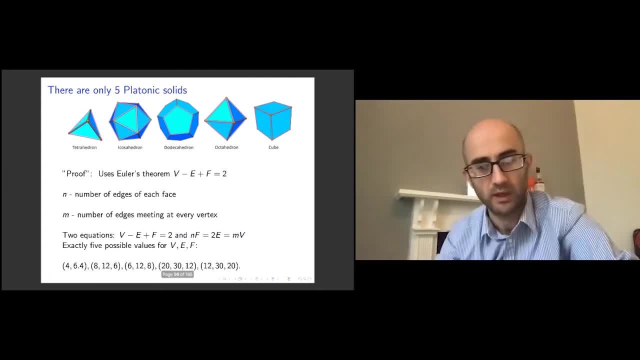 to tell you how you solve exactly these equations. And so here are the solutions: five solutions. And because you exactly have five solutions, you conclude that these exactly correspond to the five platonic solids. And these equations have five solutions, exactly tell you that there are only five platonic. 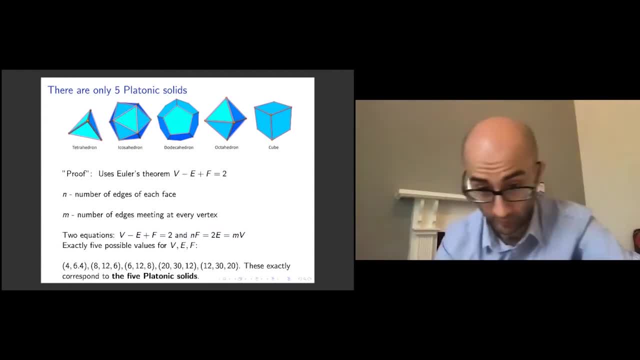 solids, And this is how often topology works. So you translate the problem into algebra, You solve it into algebra using some equations or identities, And then you go back to geometry and conclude something in geometry which is a typical way of working in topology. 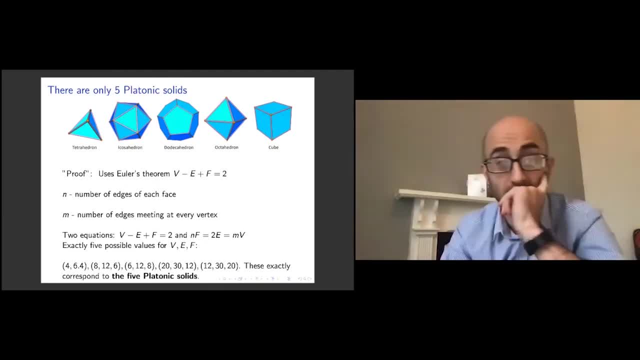 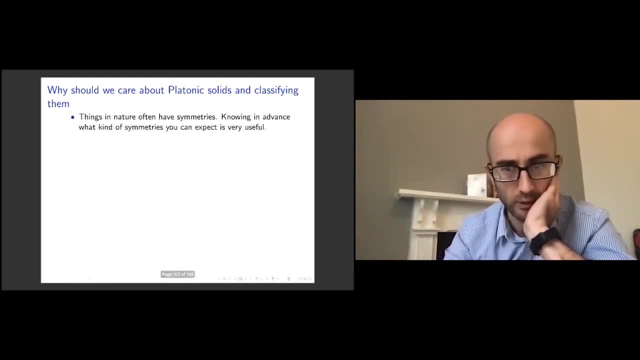 All right, So I hope you understood this. Now, why do we care about these platonic solids and classifying them? I mean, of course, things in nature often have symmetries, But we're not going to go into that And knowing in advance what kind of symmetries you can expect. 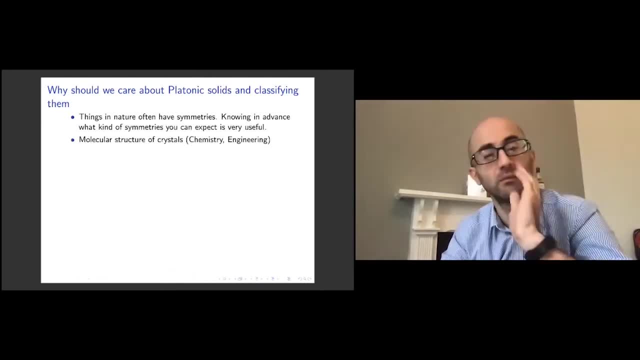 is very useful. I mean, and platonic solids are these kind of symmetric objects. They, for example, show up in molecular structure of crystals in chemistry, engineering, or they also show up as shapes of certain viruses, for example in microbiology, medicine And 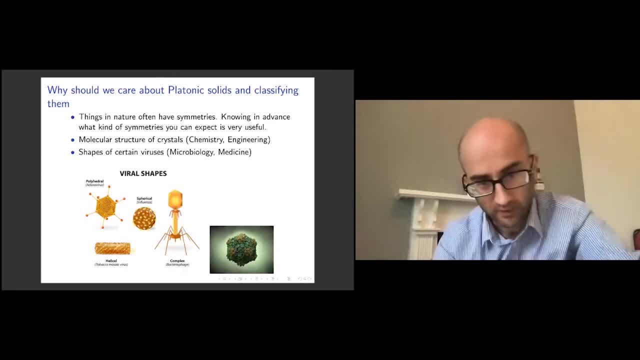 I mean, unfortunately, these days viruses are pretty important, So let's have a look. I mean, these are some viral shapes, And often these viral shapes have a form of icosahedron or dodocahedron or truncated dodocahedron, depending on what kind of viruses you have. 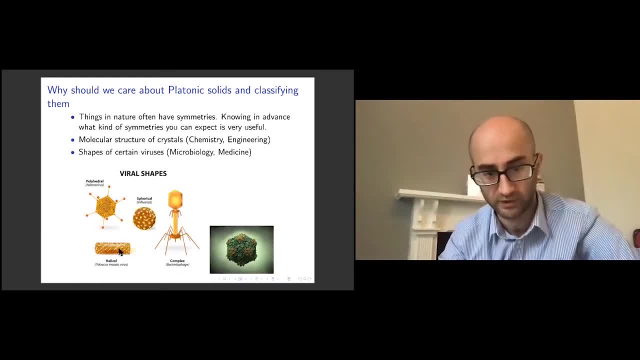 But then again, like some of the other shapes, might also show up, like cylinder we already discussed, and then we will soon hopefully discuss also spheres, And these are here, the spherical shapes. So just that you know, this talk was advertised 20 minutes, but I surely 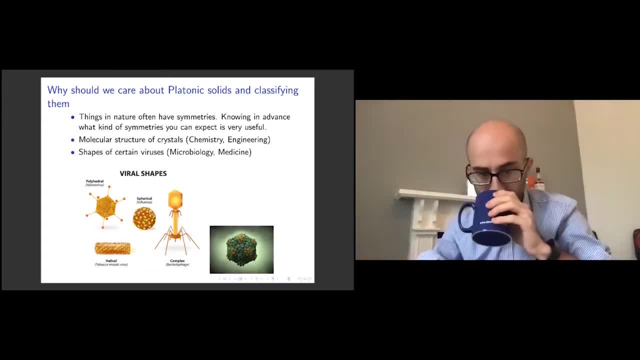 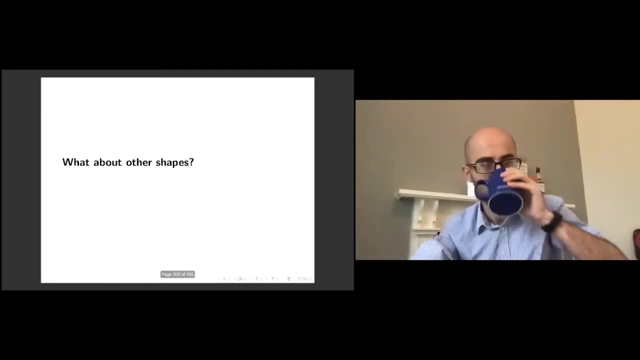 will go over time and it will be maybe another two or three extra minutes, All right. so what about other shapes? As we see, viruses also can be other shapes, So we should also study other shapes. So one of the things also topology studies are: knots Like these are also like these. 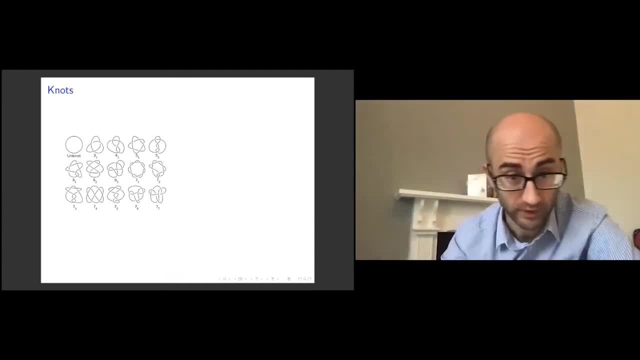 kind of you know some knots in dimension three, And so what topology wants is to distinguish these knots and stunning notes. actually probably goes again back to classical era, And this is a famous picture of Alexander the Great cutting the Gordian knot. It's a famous story. 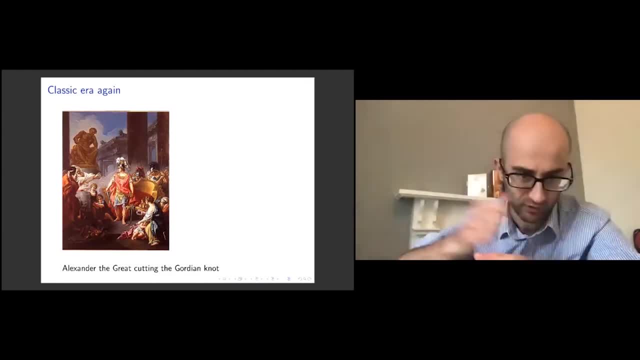 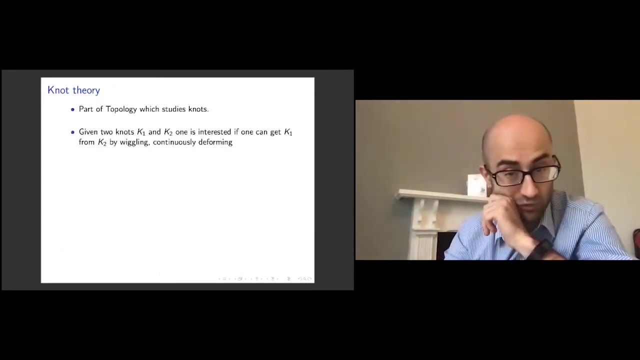 that somebody brought Alexander some knot to untangle, untwist and Alexander the Great couldn't do it, got angry and cut it with a sword. and what knot theory is about is trying to avoid that. so knot theory is a part of topology which studies knots, and given two knots, one is interested. 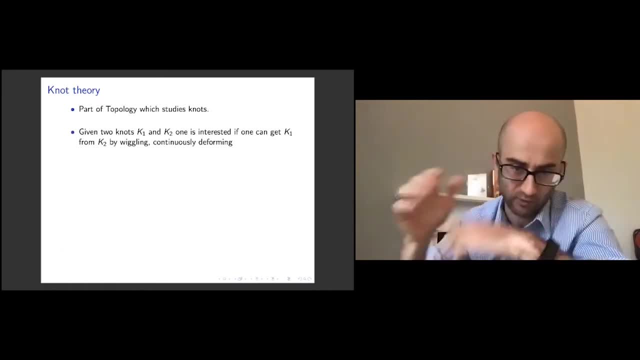 if one can get one knot from the other by wiggling or continuously deforming, uh, and cutting and gluing is not allowed. so you are not supposed to cut it and glue it back, you're only interested if you, by continuous procedure, can get one from the other. and so, alexander, what alexander did that? 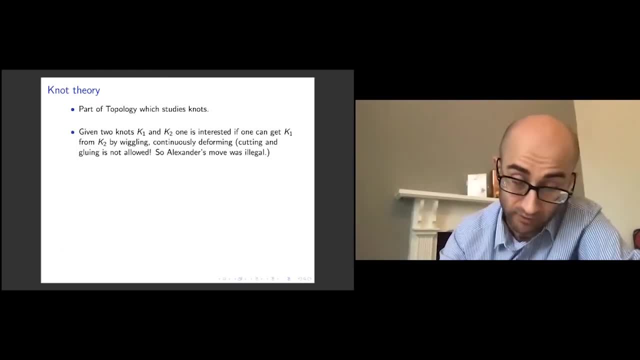 was an illegal move and not theory is trying to avoid that. okay, so what are the applications of not theory? before i tell you how exactly no theory works, it's everyday life, like you can do this in genetics as well, like something called untangling dna's. if you have seen models of dna's, they are: 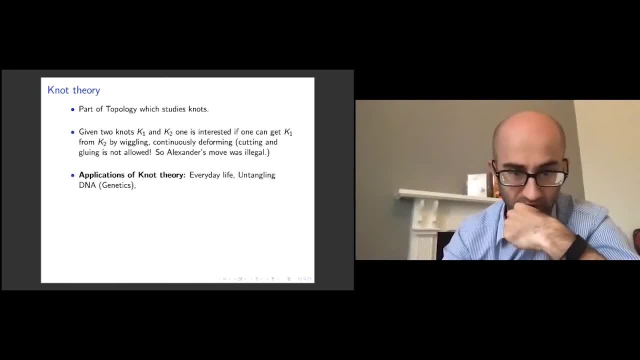 kind of not knotted type shapes. then you have quantum computing, which is in computer science an important thing, because usual computers sometimes cannot do some very big calculations. and then you need quantum computers, and these quantum computers are based on some kind of schemes which you can build, and- and this is a typical scheme for quantum 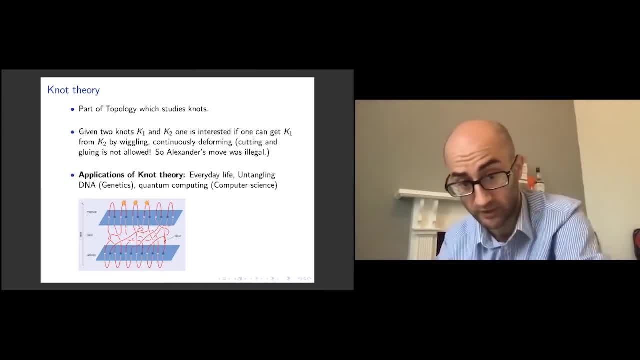 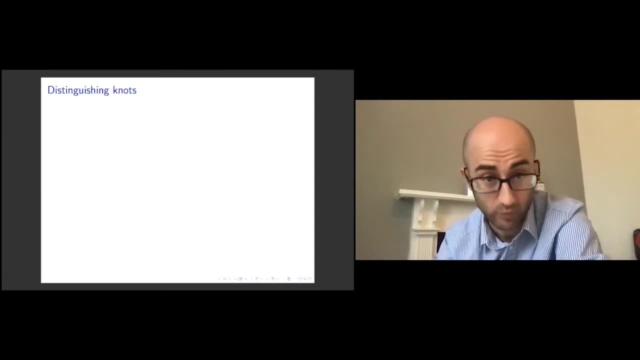 computer, and then these shapes look like knots, and then you need to know some knot theory in order to be able to operate with them. uh, anyway. so, uh, we want to distinguish knots. that's what topology is trying, and you see at this picture, for example, if you take this seven one and seven two, 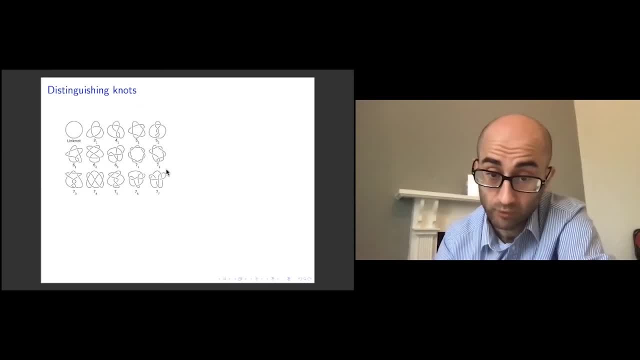 uh, then you want to distinguish, uh, these two, and how do you know that you cannot deform around that that's seven one, for example, and get seven two. i mean, it's not completely obvious. and so there was another alexander, now this time in the 20th century, a guy called jw alexander, or 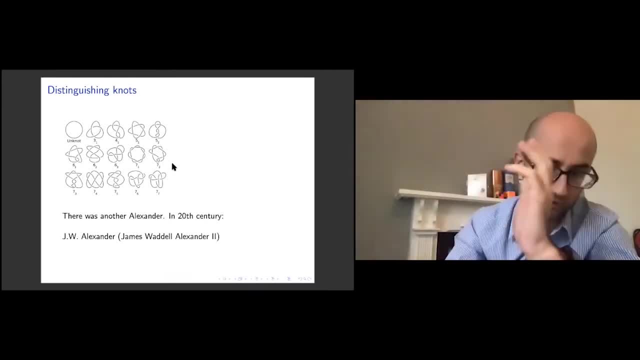 james wattle, alexander ii as opposed to alexander i the great, and this guy introduced something called alexander polynomial. i mean, we call it alexander polynomial, of course he didn't call it like that- and he associated to every of these shapes some formula called alexander. 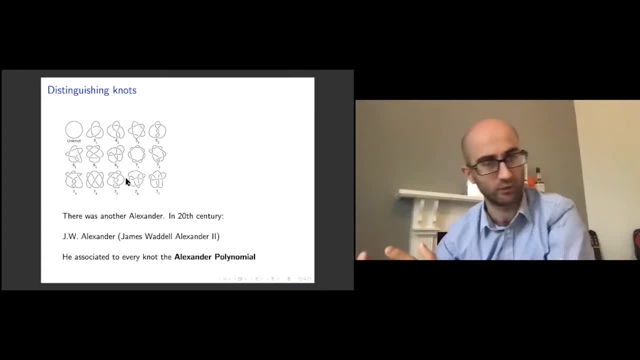 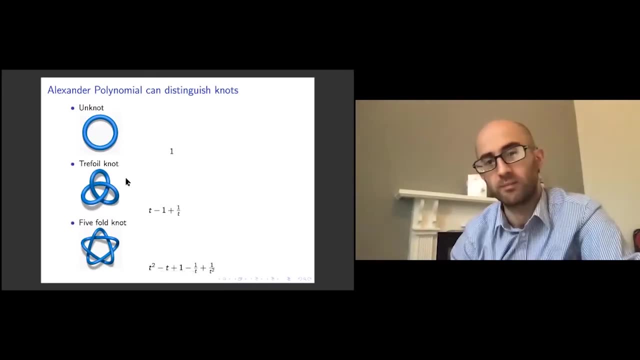 polynomial. so, given every knot, you can associate with some formula, look at the formula and then conclude something about this knot, and this is how it works. so this alexander polynomial can distinguish knots, and so for each of these knots, for example, the corresponding formulas look like this, like for this five-fold node: it's like this. and what is the point of this formula? 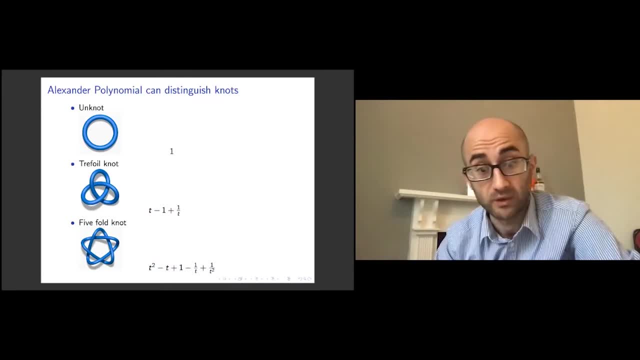 is that if you look at these, you obviously see that this formula is different from that formula and the way it works. because you see that these two formulas are different, you can conclude automatically that there is no way to wiggle around, deform this five-fold node to get a. 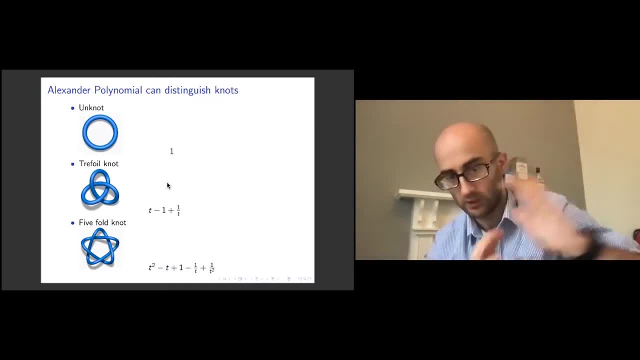 trefoil node, and that's another example how topology works. we had not theory, we had not. we wanted to distinguish them. we translated it into algebra. we see something in the algebra and now we can conclude something back in topology, uh, in geometry, all right. so now the next thing. 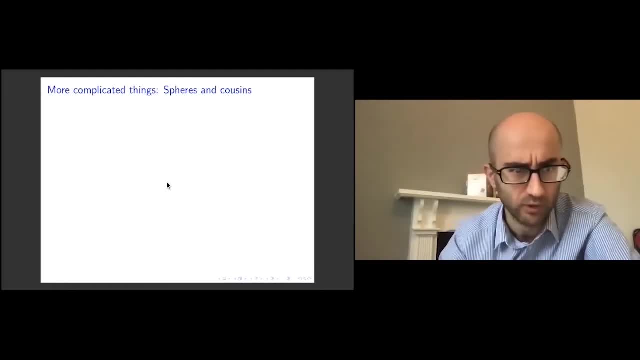 what i want to mention- and i'm already kind of running out of time so i will speed up here- so a more complicated thing. so spheres. so here is an example of what topologists like to study. these are two points. and this is a zero dimensional sphere, this is a circle. 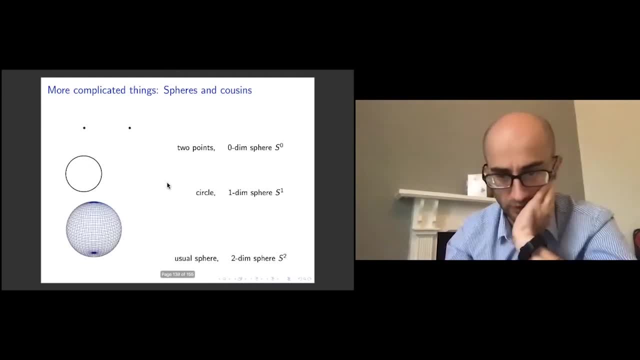 that's a one-dimensional sphere and this is the usual sphere which we call a two-dimensional sphere. and why do i mention these? because in this talk i want to end this talk by discussing something called three-dimensional sphere. and there are higher dimensional spheres- sn for nn- but in this 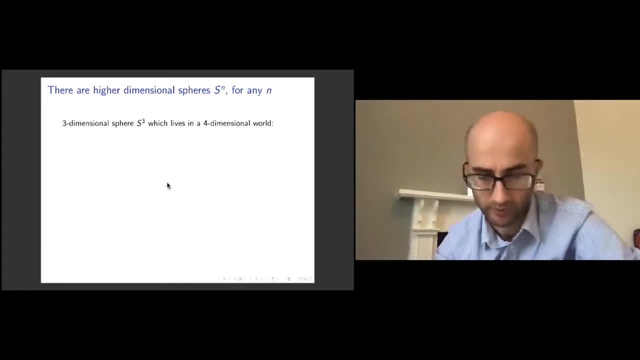 particular case. i'm interested in three-dimensional sphere, which lives in a four-dimensional world, and this is how it looks like. so a three-dimensional sphere is impossible to draw because we live in a three-dimensional world, but mathematicians and physicists, of course, imagine that they live in a four-dimensional. 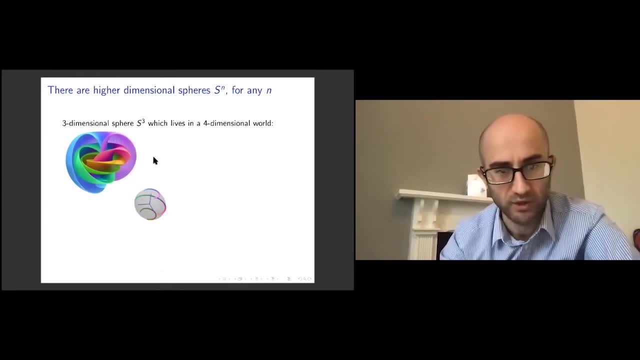 world or in any dimensional world, and so this picture here tries to draw three-dimensional sphere in terms of imagining it as a family of circles over a two-dimensional sphere. so this is a two-dimensional sphere and these points are running over it and these circles are creating here some kind of twisted shape, and locally you can sort of see it, but globally not. 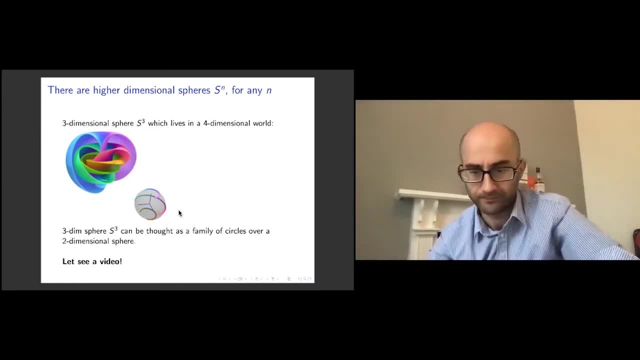 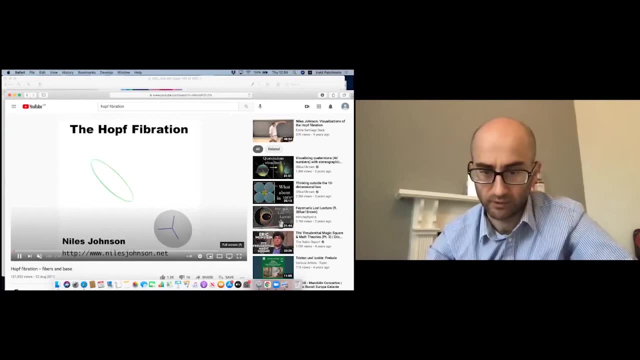 in order to better imagine this thing, we should now at the video. i have it already ready here and let me know if you cannot see it. so this is the video. uh, due to niles johnson, actually, i know. this guy is a very good topologist and very cool guy. i. 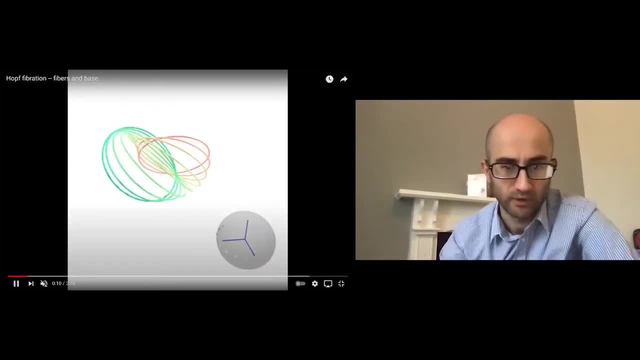 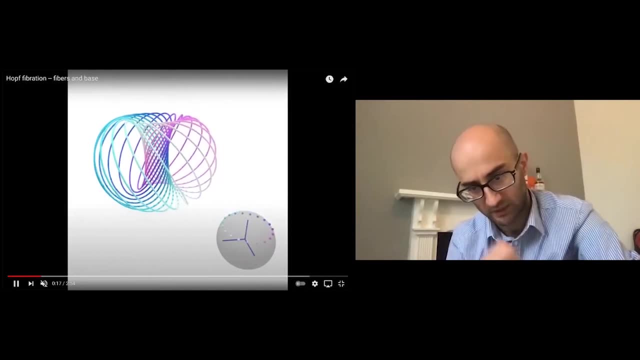 haven't met him for a while, but he's also very good at very good at making videos, and now, as you see here, this gray thing is a two-dimensional sphere and the points are running around it, and while the point is running around at every point here gives you a circle. in this picture, the 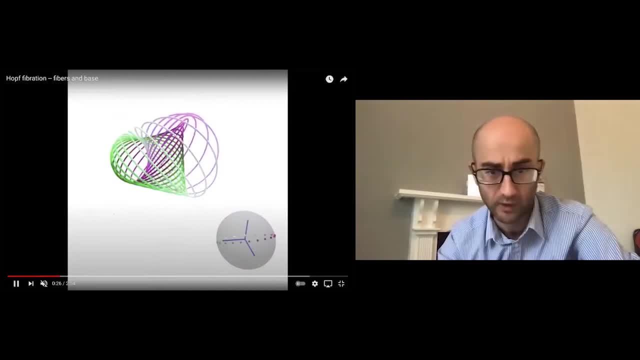 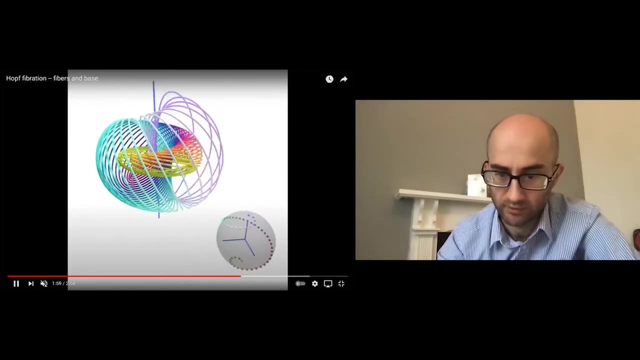 corresponding circle, and while these points are moving around on the sphere, those circles get twisted in each other and uh, and creating some funny shape. so let me go a bit farther to to make here this thing even more crazy. so, like this is how it goes, and then things become even. 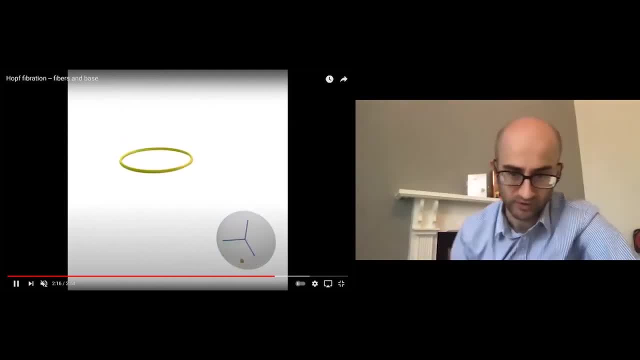 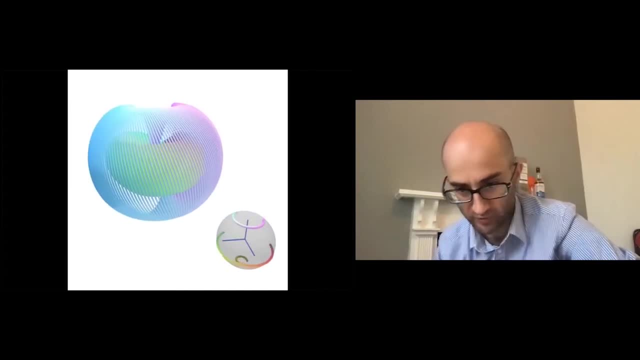 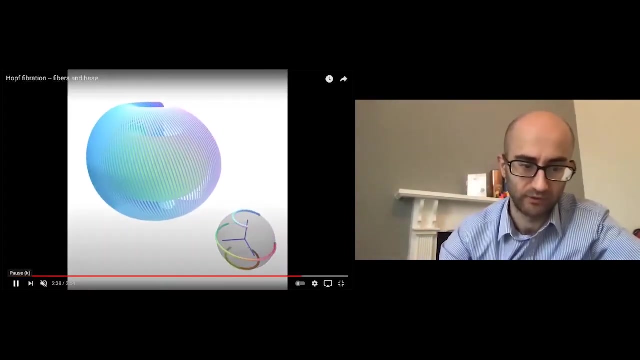 crazier after this point, and let's see that, and then you're gonna see the picture i have drawn. so this is how the three-dimensional sphere is created: using circles corresponding to points running on a two-dimensional sphere. all right, so we can now stop this video and go back to the last couple of slides i have. 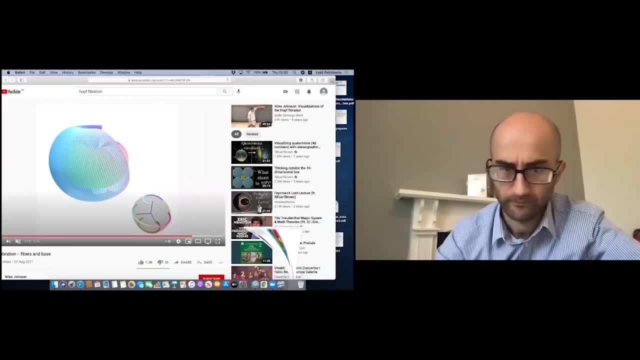 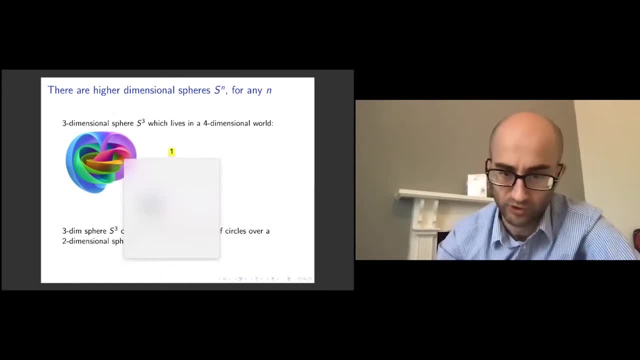 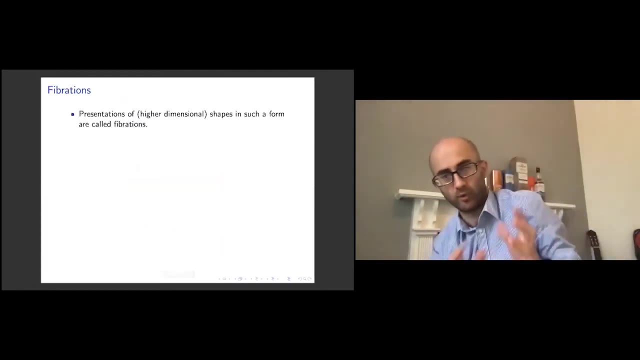 i have left um and i'm already quite over time here, but like i just like, want to finish it in a reasonable way. so this procedure, what you just saw, this is called, uh um, vibration. so this video, what you saw, is a general phenomenon, a presentation of shapes in this form. 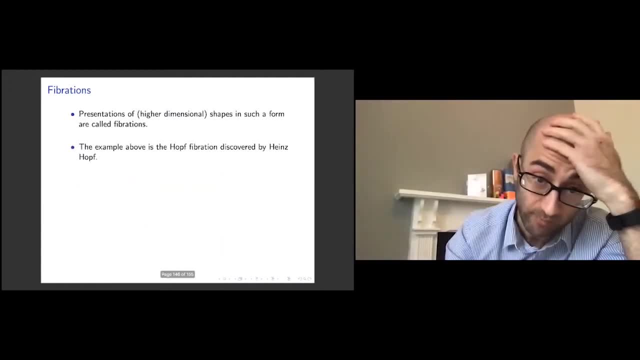 are called vibrations and, uh, these vibrations, this, this particular example, is a hop vibration discovered by heinz hop. and just that you don't think that this guy, like me, is always just drawing pictures and looking at videos like this video, what you just saw is this formula. i mean what? 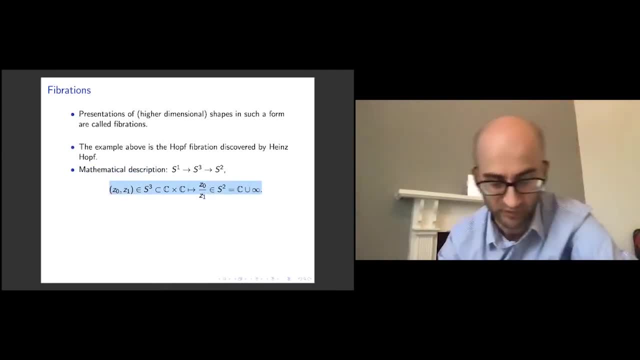 we really work with are these type of formulas and not those kind of videos, of course, but that you can ignore if you don't like formulas. and so one of these people is, you know, the guy named the most serious tasks of modern topologies- to study such vibrations and use them to understand. 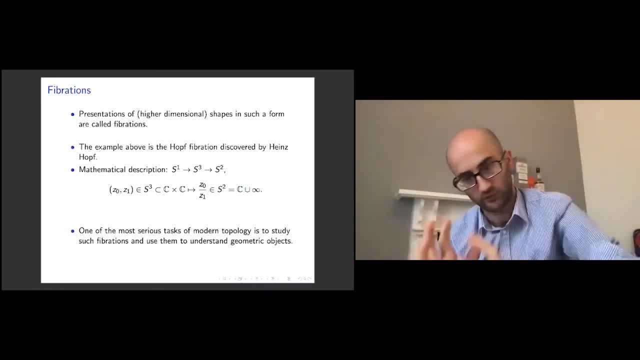 geometric objects. now this video, what you saw is a special case of some structure that shows up every day, basically in a topologist's life, like, for example, yesterday i was struggling with some vibration, which is probably a more complicated vibration than the one you saw. and okay, now 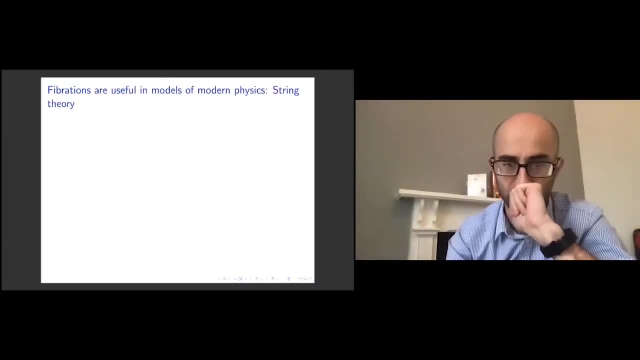 because i'm extremely over time. uh, this is the last slide i have so that you don't get scared. so these vibrations, like these kind of video, what you just saw- these kind of structures are very useful in modern physics, for example, in string theory. like this is something you saw. 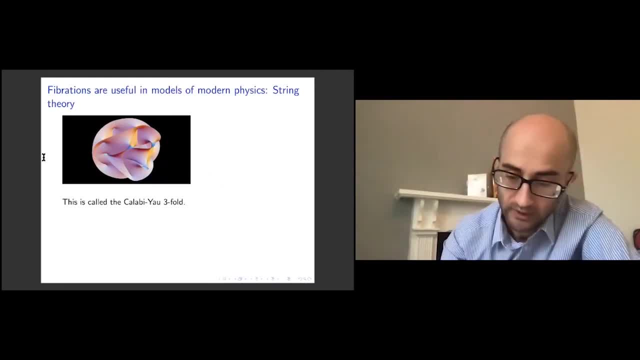 at the beginning of this talk. this is called calabial threefold, and why is this important? this is something six-dimensional, and what you just see here is projection in a three-dimensional space, and it turns out that there is a vibration, like this type of video, what you saw, but instead. 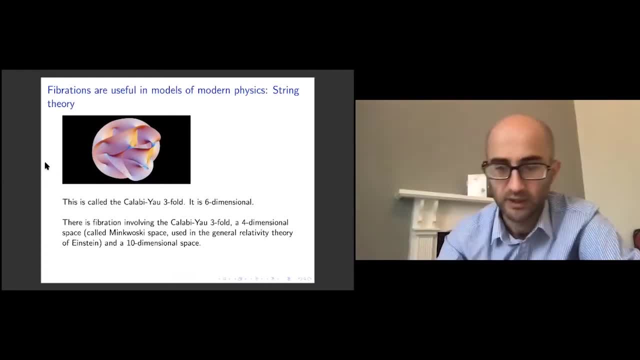 of circles and spheres. now we have a three-dimensional space and it turns out that we have this crazy gadget and we have a four-dimensional space called the minkowski space, used in a general relativity theory of einstein. so einstein's theory is four-dimensional, as you. 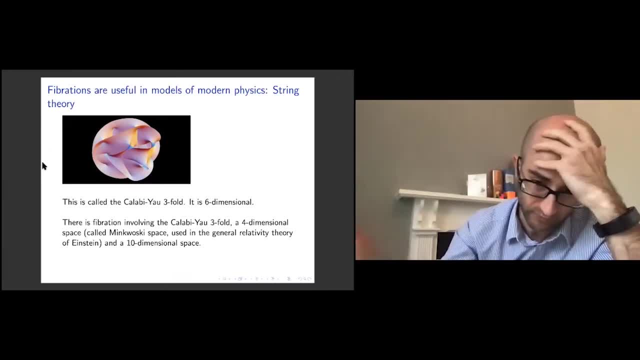 know, the fourth dimension is time. and if you take instead of this two sphere the four-dimensional einstein's relativity theory and you take instead of circles this six-dimensional calabial threefold and you, then you have some kind of vibration, so you can make a mix out of these two and then you 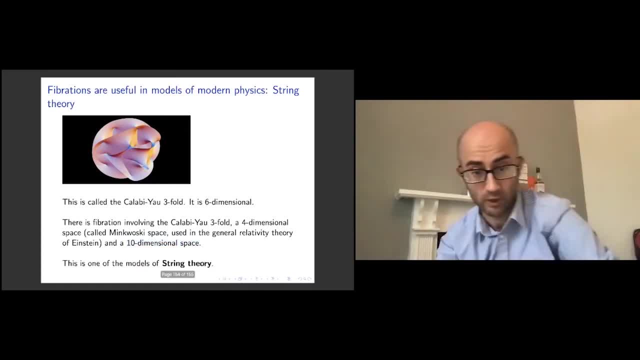 can make a ten-dimensional space out of that, and that's the model of one of the models of string theory. so string theories tell us that the world is ten-dimensional and and the and the world is a mix of einstein's relativity theory and something six-dimensional, some extra dimensions. and what is this mix? this? 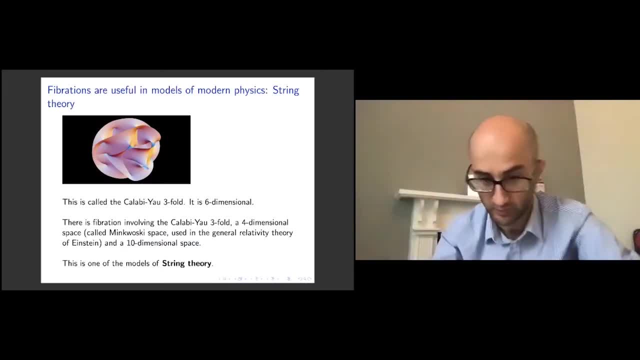 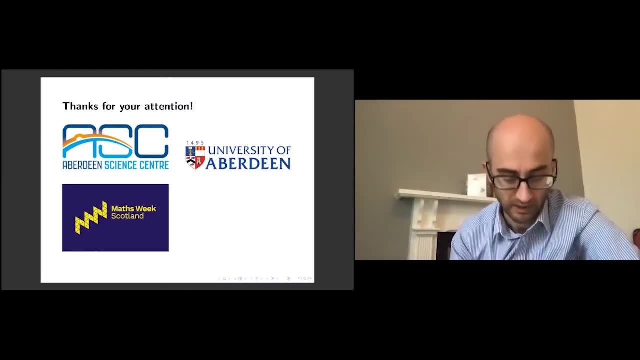 mix is exactly this vibration, the type of thing, what you saw in the video. uh, all right, so i think this is all i wanted to say thanks for your attention, and i just want to thank aberdeen science center and india, copeland and debbie mothers, and also maha bishak for organizing this. 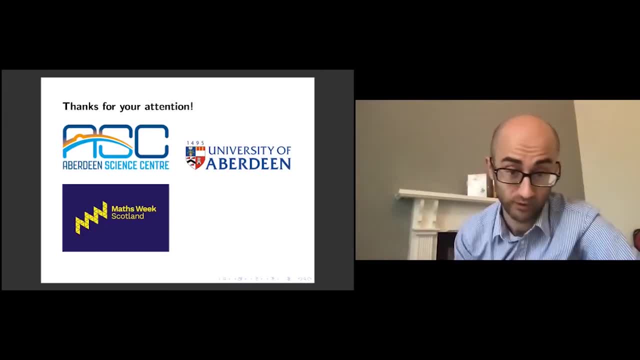 event and setting up all also maths week scotland. i would like to thank them for making us aware of these kind of events and i would like to thank my university and my math department for encouraging me to do this thing. and i'm sorry for going, i think went five minutes. 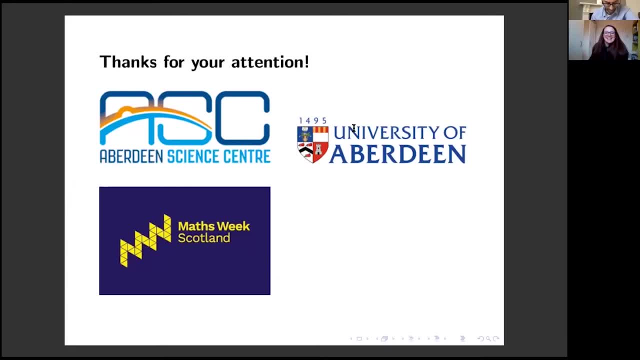 or something all the time. so sorry for that. thank you so much, iraqli. thank you very much. yes, if we can have a little round of applause on our with our reactions, that would be fantastic. thank you so much. um, nobody's left, so you're good with time. you're good with time, don't worry about. 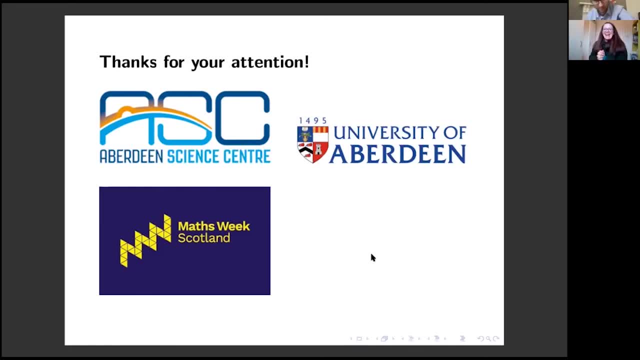 that at all. maybe they just turned off my sound. it's important, um i would like to to welcome anyone to ask any questions. you can either pop it in the chat or you can unmute yourself and ask a question. um, it can be based around what, um, what iraqli's been talking about, and i'm going to. 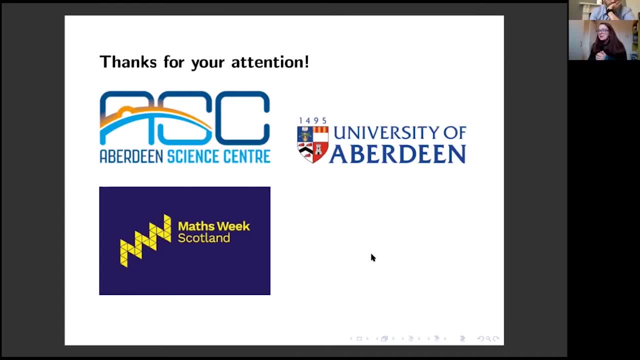 or maybe he can take a punt at some other maths related questions, but i don't want to promise that from him, um, so yeah, is anyone any questions at the moment? maybe, while people are thinking of questions, i'll um, i'll pop one in. um, how did you end up studying topology? oh, that's a good question. 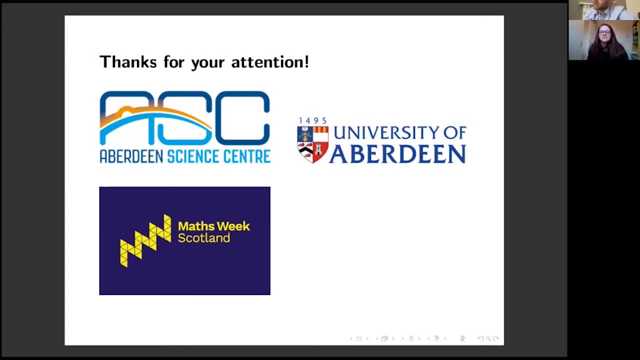 so i mean, i think one of the reasons why i ended up studying topology is that i had this book as a school, um, in the school, in the high school, something called uh, something called what is, what is mathematics, or something like. i forgot it. this famous guy called kurand who wrote that book. 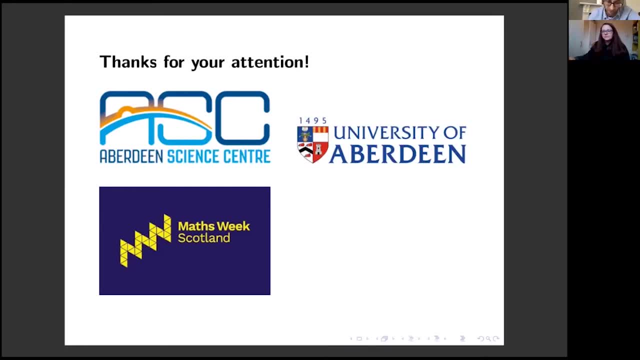 and i remember first time my encounter with topology was to see these pictures in in that book. so i got really interested what these pictures were. but then the reason why i actually ended up with topology is something more abstract. so there is a foundational aspect of this topology. 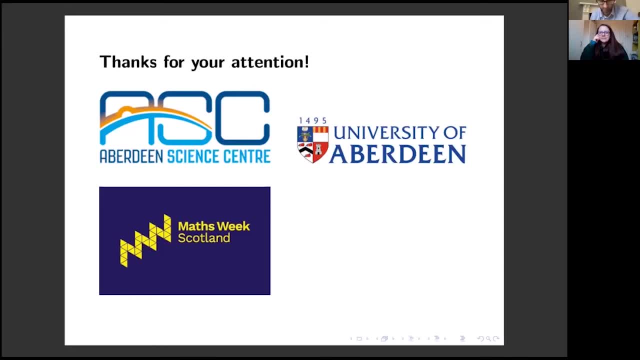 called poinsett topology, so which is not based on pictures, and as a, as a student, i really liked this subject because it was very clean subject. somehow it was describing all these geometric phenomena completely in terms of math, without ever doing anything geometric, and so i understood that. 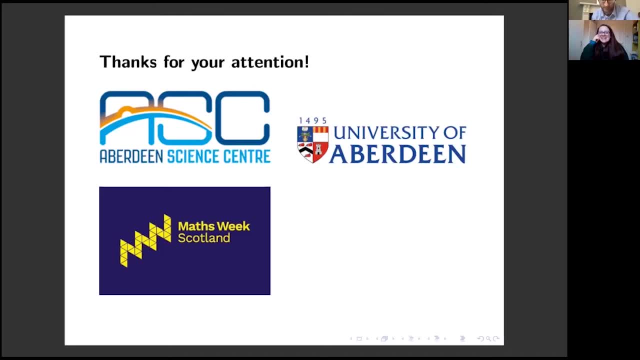 like, okay, all these geometric things, they look cool, but there is a way actually to do these in a very clean, formal way. and i guess is that the kind of thing where you were saying, where you then move into algebra to sort of do this and then you're like: oh, i don't know, i don't know, i don't? 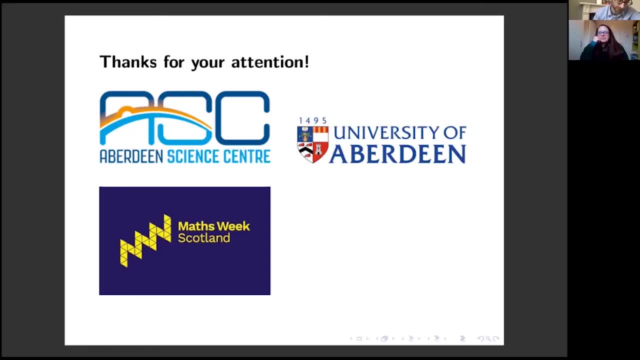 know exactly, exactly so. so this is why i ended up doing this kind of thing. like you have this very geometric thing and you don't want to really mess around with geometric figures. instead, you translate it into algebra and then you would do things there, and then you come back somehow and do geometry and 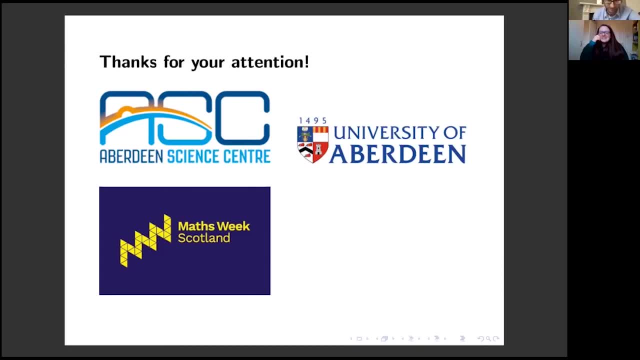 sort of you actually did much cleaner work in algebraic side than then onto on the geometric side, and that's sort of like why i got interested in this. that like there was a way of actually doing these very difficult geometric things in terms of algebra, that was kind of that was kind 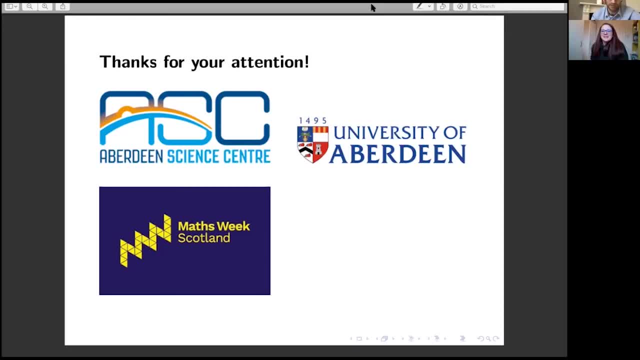 of cool, yeah, okay. yeah, we've got a couple of questions in the chat, so lindsay's asked um. what sort of research do you do um, and could it be used for code breaking or encryption? uh, oh, yeah. so what kind of research? i mean, i do a lot of research in this topology, so, like for 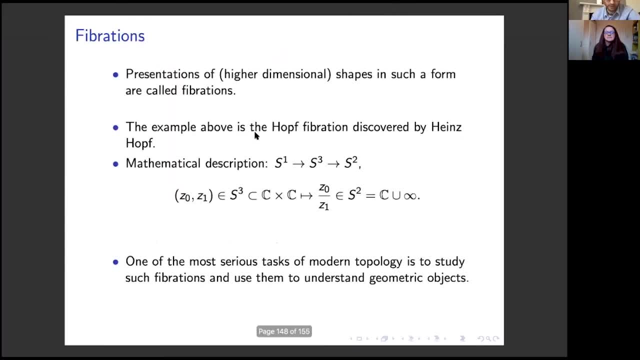 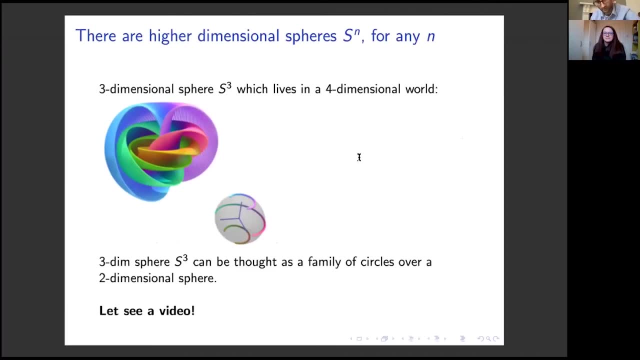 example, these vibrations, like- let me go back to this thing- like these type of structures, these vibrations or like these kind of things. so, uh, we try to do is that? i mean now, if this was a simple example, we have sometimes way more complicated objects. we want to understand which motivation for studying these objects again could. 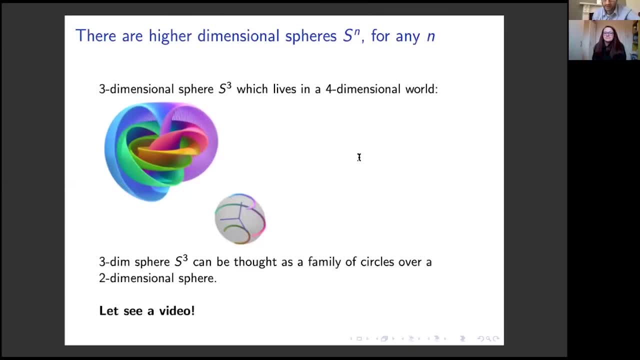 come from physics or many other things, and it turns out that it turns out that that studying these kind of shapes requires some technology, like, for example, these vibrations. and then you want technologies that study these kind of vibrations, and one of the things what i research, for example, is is: is these kind of vibrations or things that can be used to say something about? 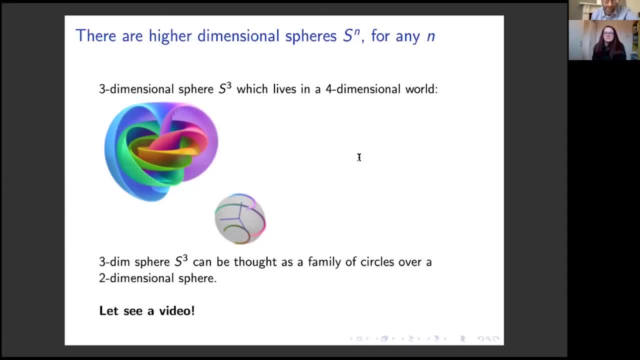 these kind of vibrations and also just using these vibrations in other type of problems of topology and so on. so it's studying these kind of geometric objects, but also higher dimensional ones, for example. you know, like it doesn't have to be as i, as i was mentioning it was a six. 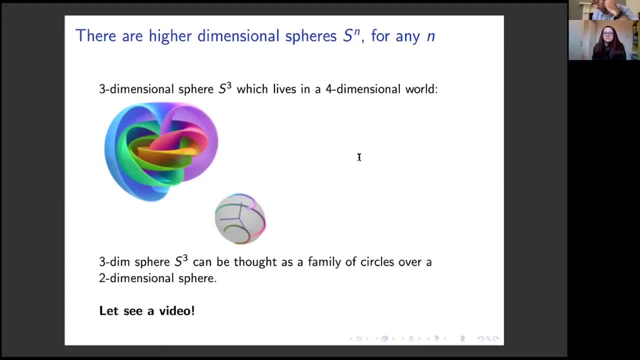 dimension, ten dimension and so on. so, like the area which i work in is called homotopic technology and that is the type of stuff that i am studying now. so i'm trying to learn from that theory and that most studies like studying these kind of objects up to deformations. 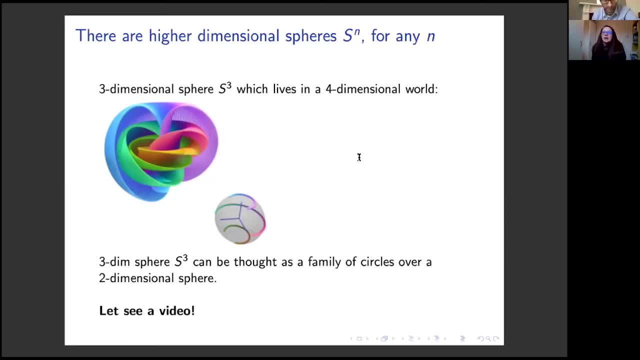 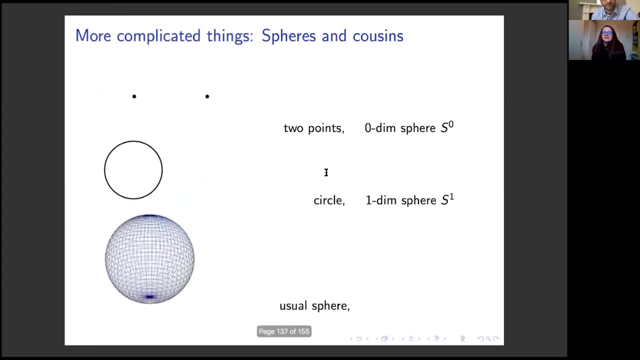 and and i also do a lot of algebra, because a lot of algebra is motivated by these things and and then you have to do a lot of algebra as well. now another question: what about encryption kind of stuff? right, the codes and stuff that is related to not theory actually. so let's go back. 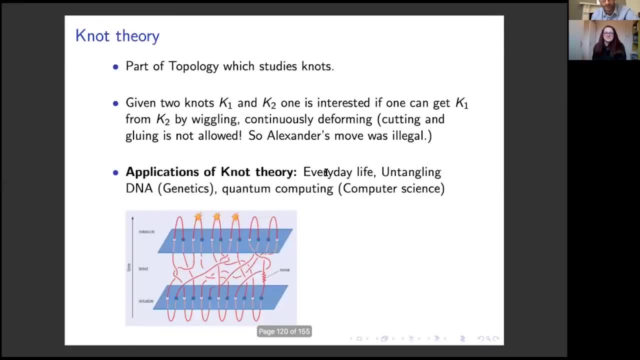 to this quantum computing business. yeah, so this quantum computing is something that that does rsa algorithms that's used in cryptography, for example. so so you have some ways of encrypting some kind of things and there are some big numbers you have to use for this and this quantum. 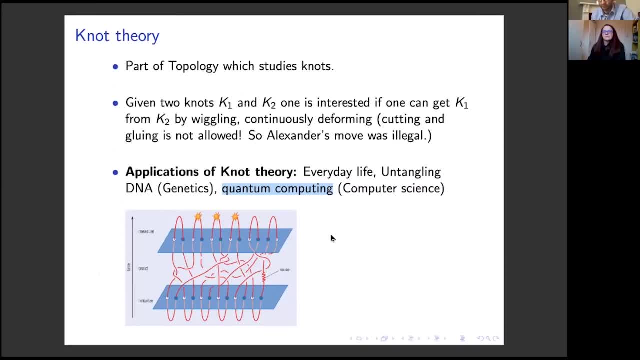 computing, for example, is, uh, is very useful for that. yeah, so i hope this answers at least a bit you, your question, yeah, oh, and i think as well i remember you saying that, um, your research is very theoretical, um, and not not applied, so maybe the stuff that you were doing at the moment won't. 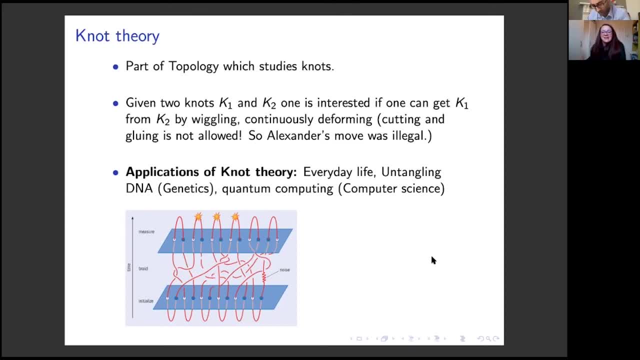 be used, right? yeah, it is right. i mean, of course, like actual current research i'm doing is very abstract, but you know, like some of these things i was talking about which are nowadays used, maybe 50 years ago or 100 years ago was also, uh, considered. 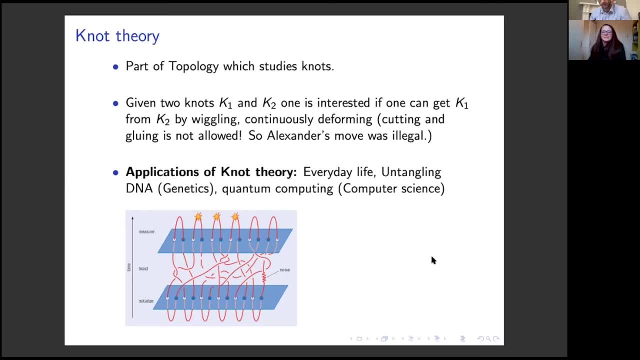 to be very abstract, but then eventually they all got used in uh, in in technology and these kind of things. so so yeah, i mean mostly the research i'm doing is pure fundamental research and it probably will be uh later used, hopefully some of it. yeah, i see some questions. i was going to say 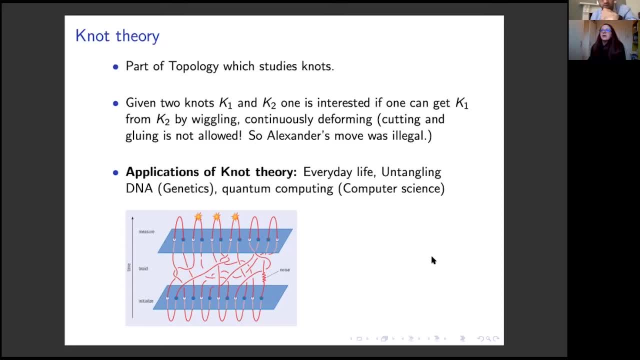 the other question we've got um is: could you give us a quick idea of what homology is? uh yeah, so one of the ideas of homology is that, like, imagine you have a surface or something which has holes in it. so what homology is really does is the way to count these holes. like, for example, you have a. 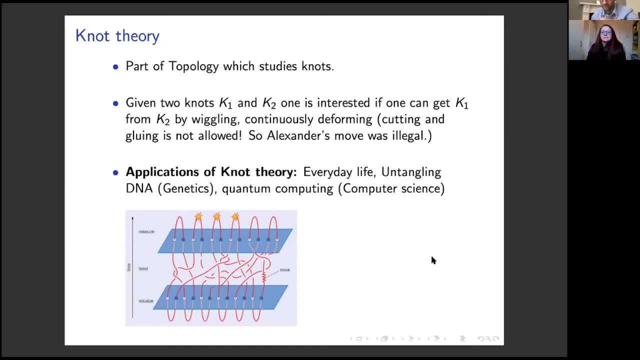 torus that has one hole. homology would see that. and so if you have like some object that has, like say, four holes and the other object that has five holes, then you're gonna sort of capture the difference between these two. of course, you see that these two things look differently, but what's? 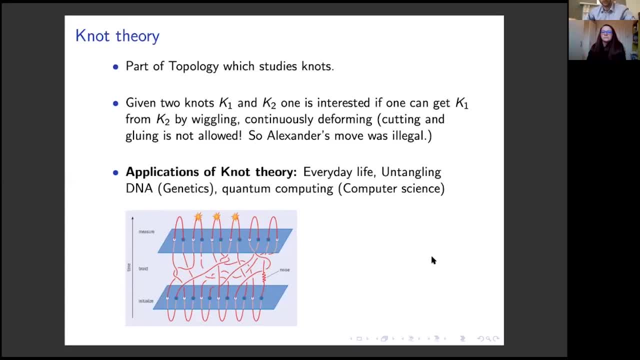 the mathematical way of distinguishing them, and that's what homology does, sort of seeing those, these, these things that how, like, what's the genus somehow, of this uh, of this surface, for example, is seen by, uh, by homology. like homology is going to distinguish between disc and circle, because disc doesn't have holes in it, whereas 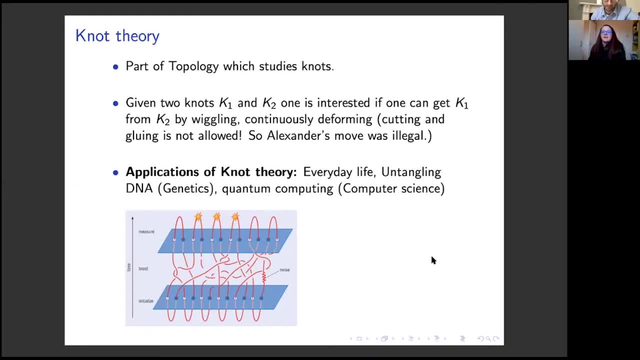 circle was just something in a, in a sort of a tube shaped kind of thing, right, so so, uh, yeah, that's what homology does distinguish. i'm just while sorry, i'm just i'm just aware that some people are popping, popping off the call and just before everybody leaves, 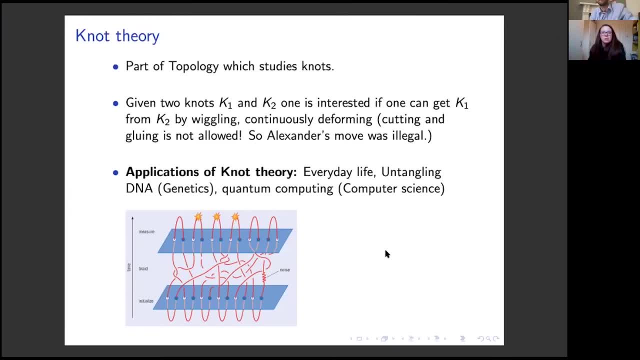 i'm just going to launch the poll. we'll still keep answering questions, but it would be great if you could just uh answer. answer the poll, just so we can get a little bit of feedback. and india is also going to pop a feedback uh link in the chat to get a bit more in-depth feedback. 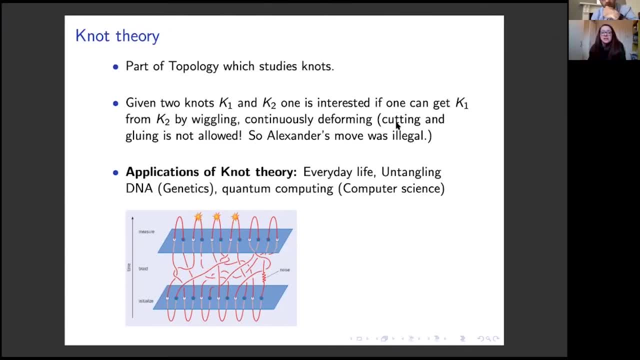 and it would be great if as many people as possible could fill that in, not just for the science center to improve um events like this, but also for erratically to to know, uh, what you and what you'd like to hear more about. so i'm going to keep that open but, as i said, i hope that. 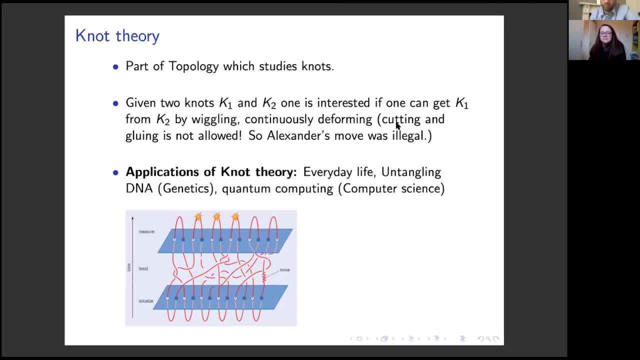 stay in and answer this answer. what i gave, i hope, about homology, that was okay, i hope. i mean, i don't know if. i mean, if you want to study more homology- and i see who is asking this question- uh, you got to attend the algebraic topology class of the fourth year, you know. so, um, so the other question. 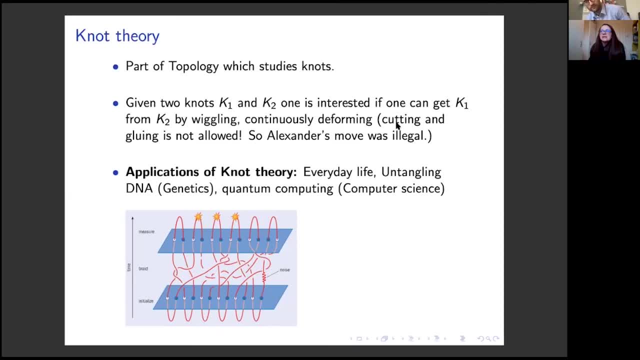 we've got is: are there other ways of distinguishing between knots besides alexander? definitely so. alexander poli was the first one that was invented. there are much better ones that can do this. there is so-called jones uh. there is so-called jones polynomial uh, which is much better way of distinguishing, uh. 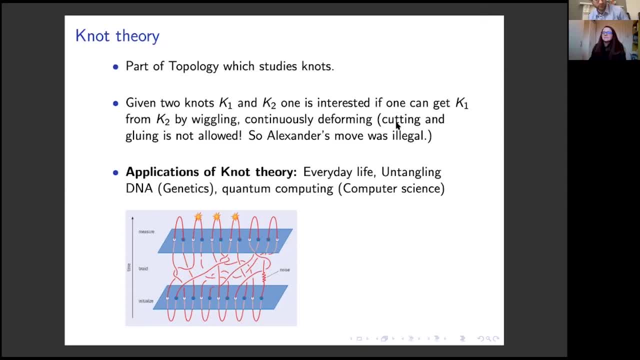 uh, distinguishing knots, jones polynomial is even a better invariant, which is the complete invariant somehow. i think, uh, like two knots are equivalent. i think if and only if they're, jones polynomials are equivalent as far as i remember, or maybe i'm wrong and just, but very often it's the better invariant, yeah.